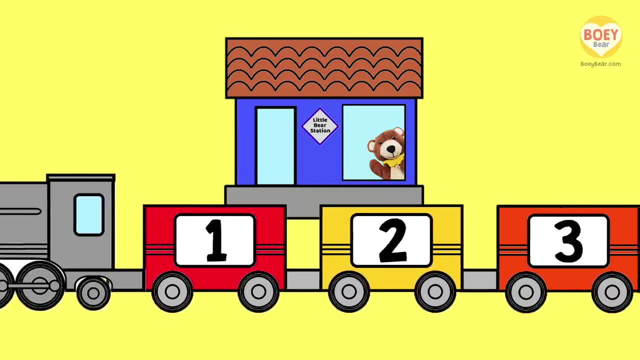 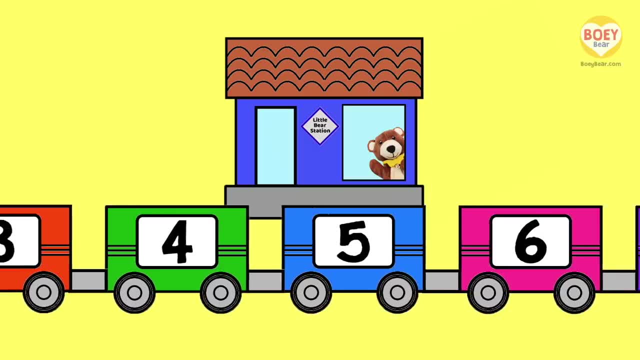 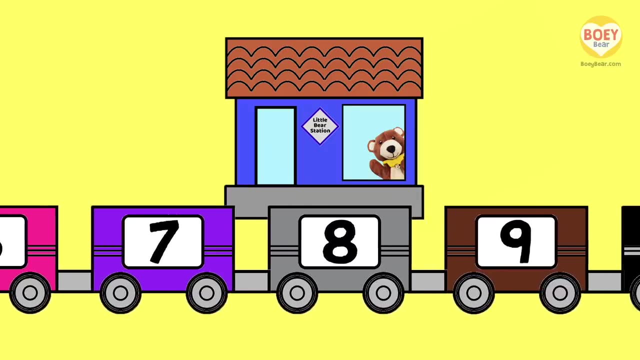 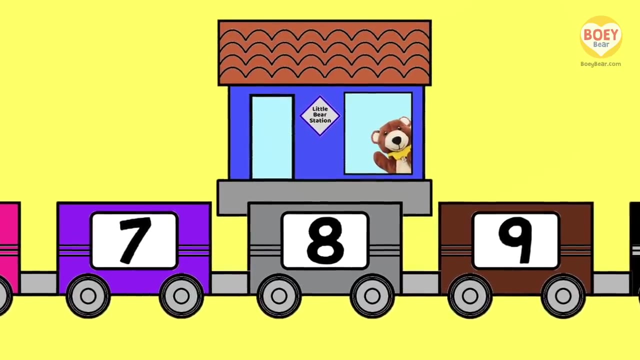 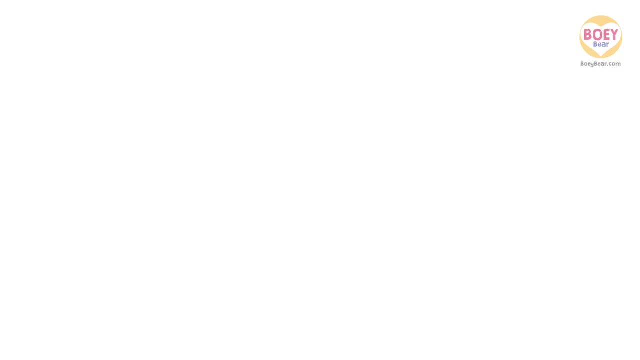 One, One, Two, Two, Three, Three, Four, Four, Five, Five, Six, Six, Seven, Seven. Ooh, It's slowing down. Today's number is eight. Can you say eight, Eight, Great, Okay, everyone, we're going to jump eight times. 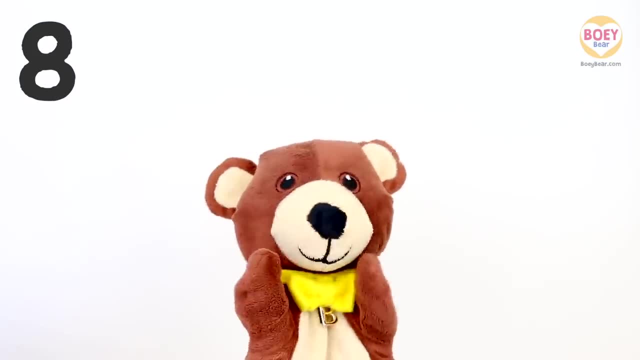 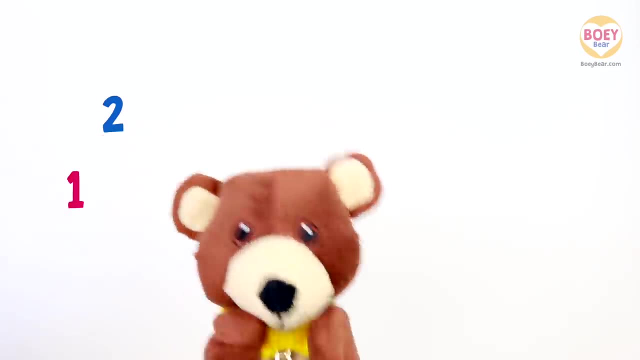 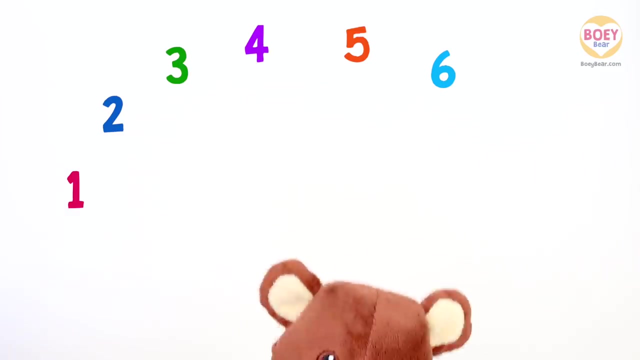 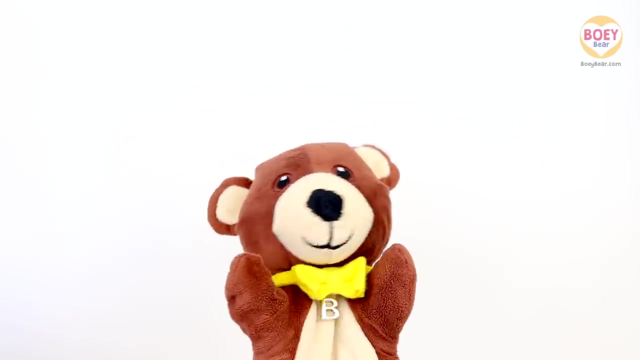 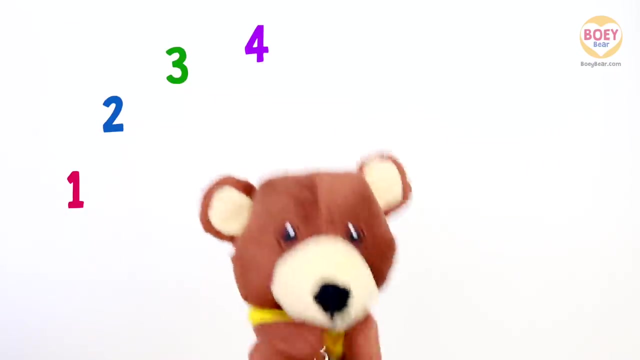 Ooh, Stand up at home and get ready to jump Ready. Go One, Two, Three, Four, Five, Six, Seven, Eight And again. but jump faster. Ooh, Count as you jump. Go One, Two, Three, Four, Five, Six, Seven Eight. 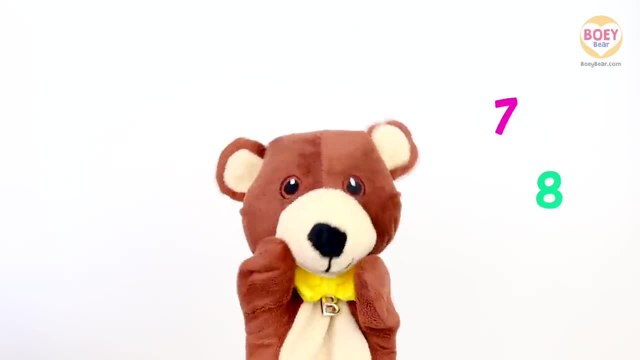 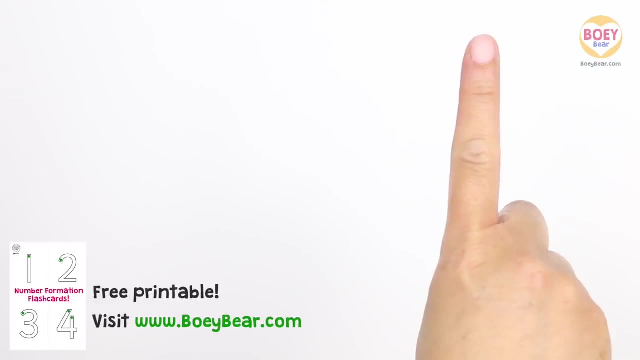 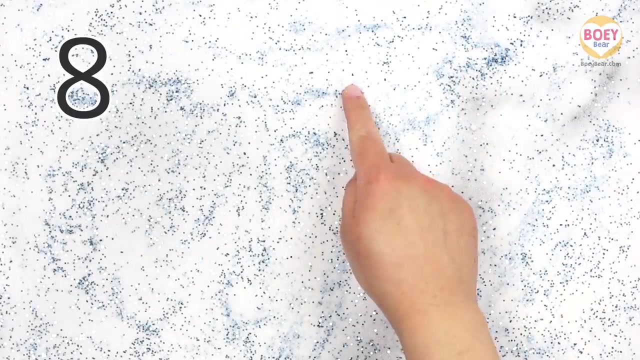 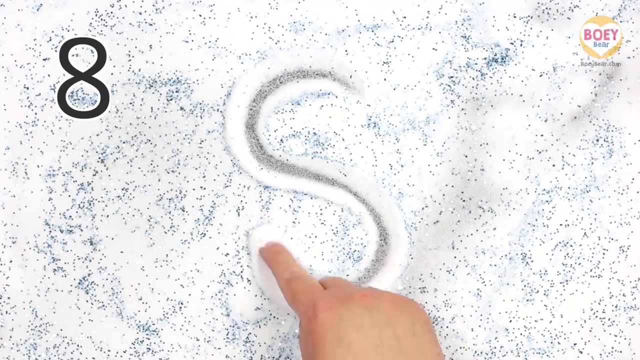 Well done. Yay, We jumped eight times. Here's how you write it. Get your finger up in the air and copy along: Ready Steady, Go. Start at the top Curve, round like a snake, Then cut through the middle and round back to the start. Let's do it again, but 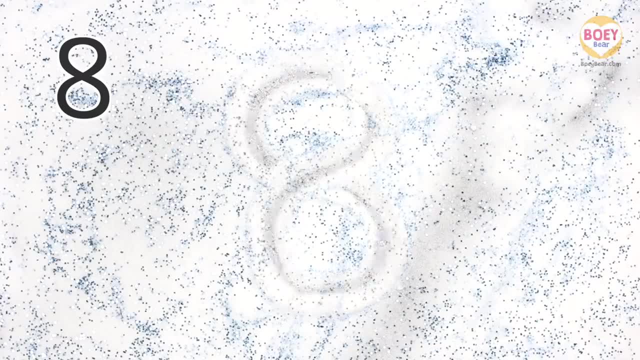 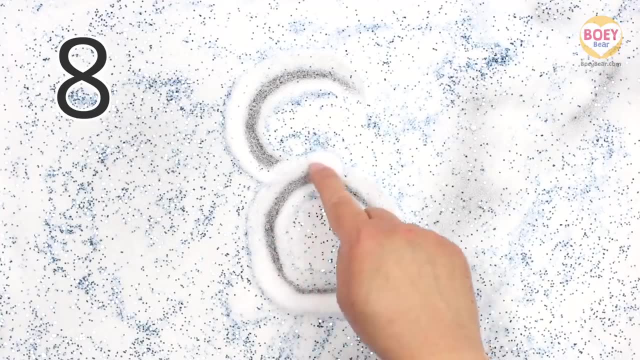 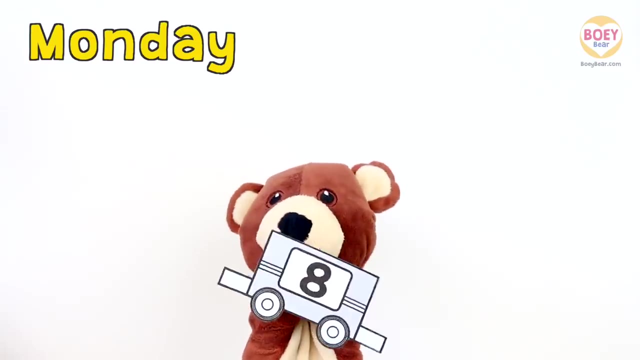 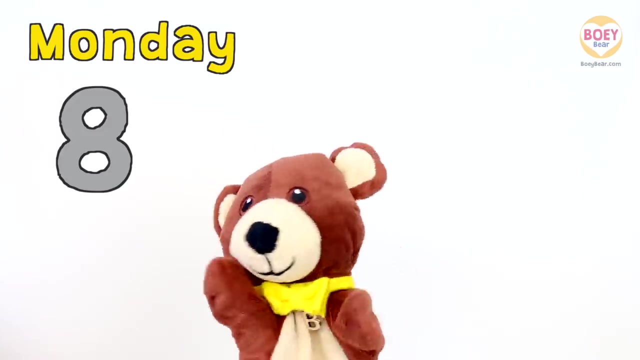 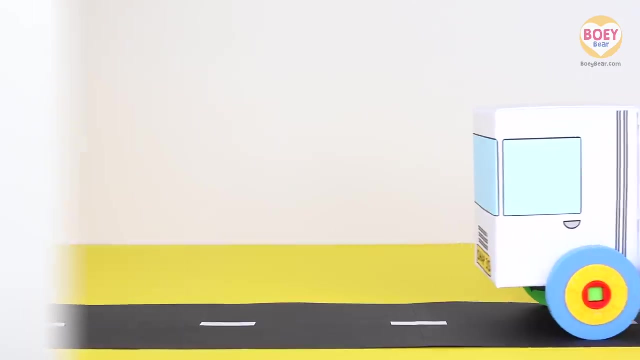 a bit faster. Copy along with your finger in the air: One, two, three, four, five, six, seven, eight. Well done. Today's number is eight. Yaaaay, Can you hear that? Ooh, What's that? 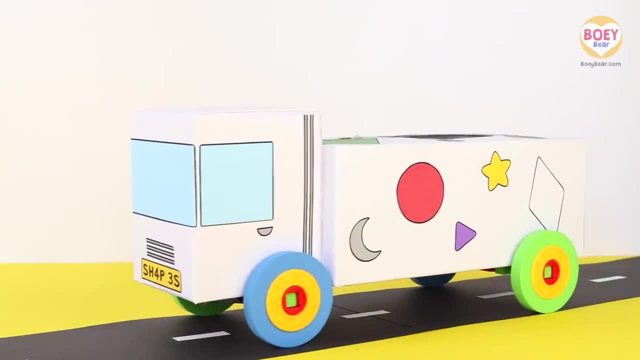 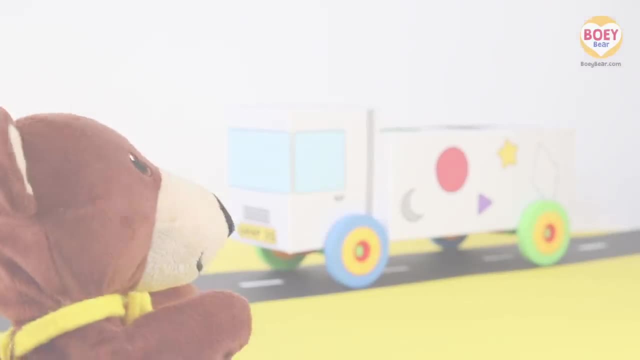 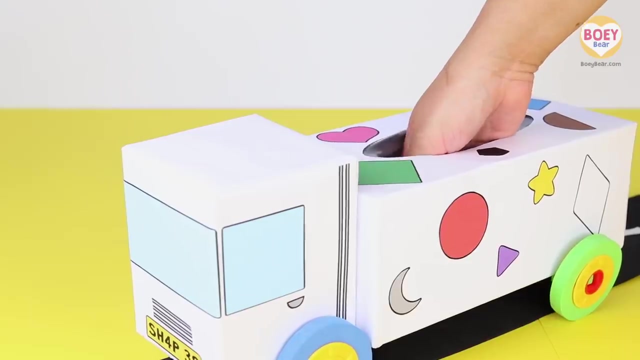 It's a rocket. It's the shapes truck. I wonder what shape is inside. I'm going to put my hand in and see what shape we have today. Hmm, it has two curves that meet at a point at the bottom. Can you guess what shape it is? 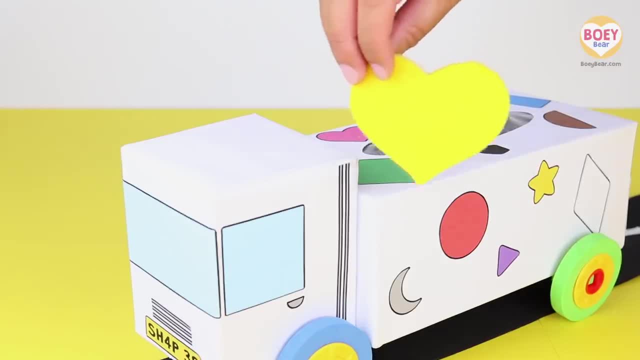 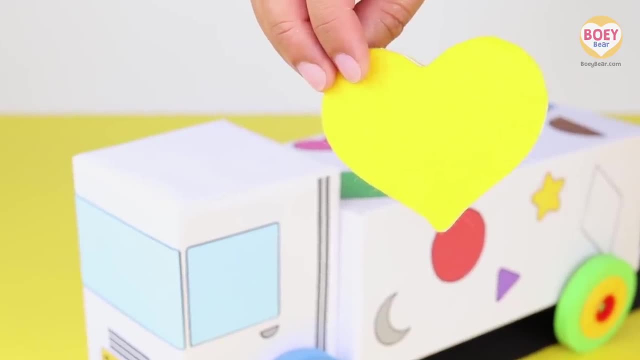 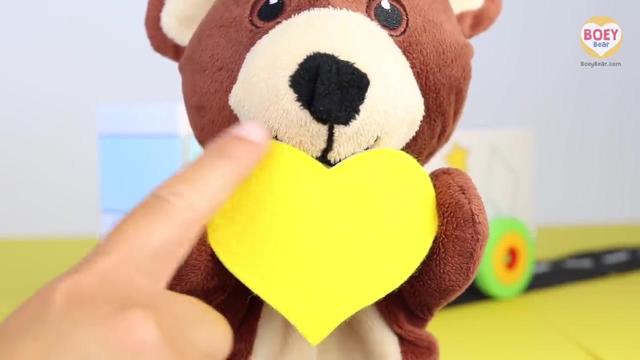 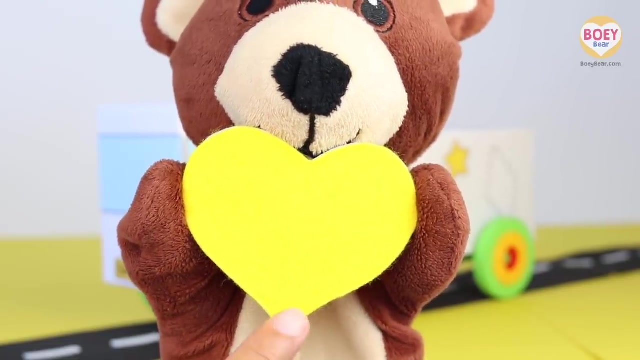 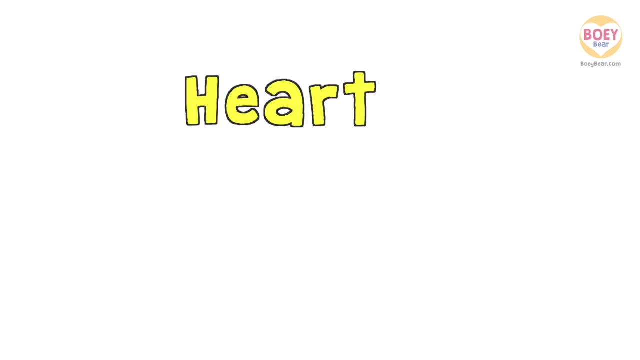 It's a heart. Can you say heart, Heart, Great. It has two curves, one, two that meet at a point at the bottom. What things around us are? a heart shape. Get ready to answer. A heart shape Necklace. 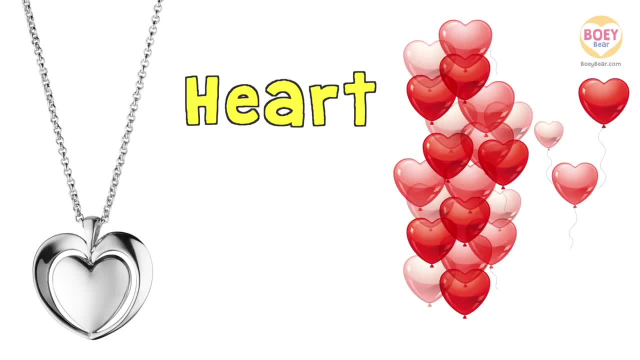 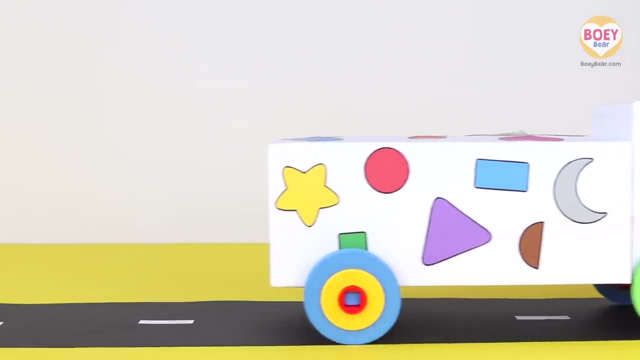 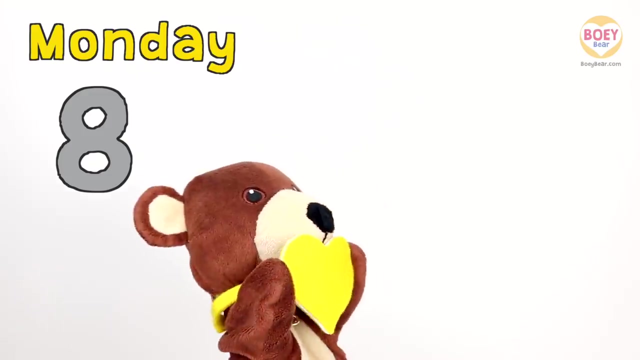 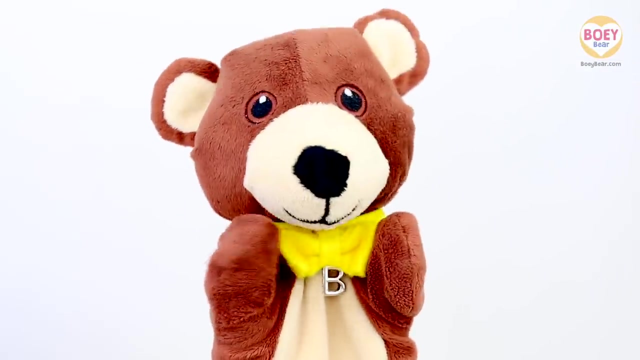 Heart shape Balloons And a heart shape Rock. Great, Thank you shapes truck. So today's shape is a heart Roll, roll, roll. Yay. Was that your tummy rumbling Bowie? Was it your tummy at home? 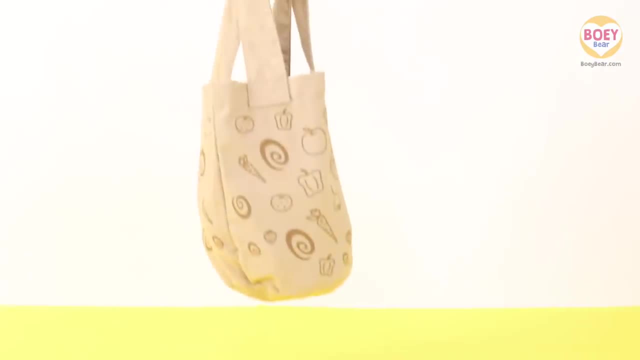 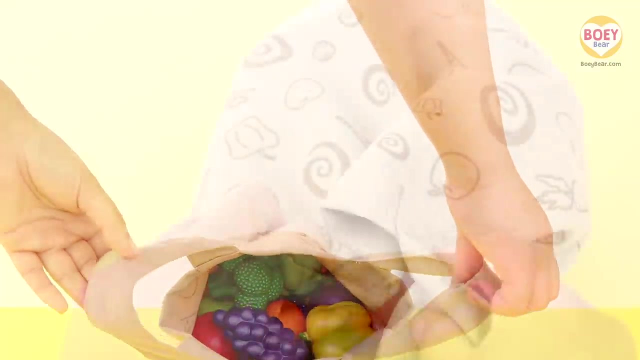 Oh, it might have been mine. I think we're all hungry. It must be snack time. Here's my grocery bag. It's full of different fruits and vegetables. Have a look, I'm going to pick this up. Here's a snack. 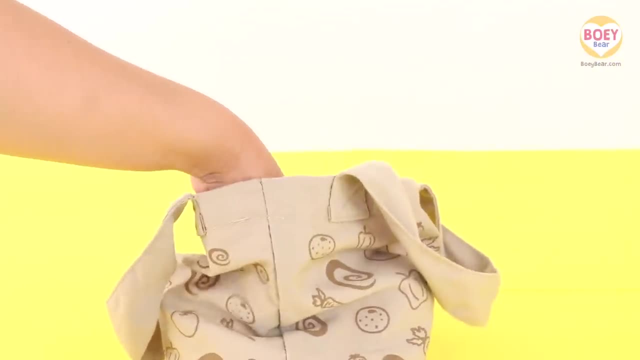 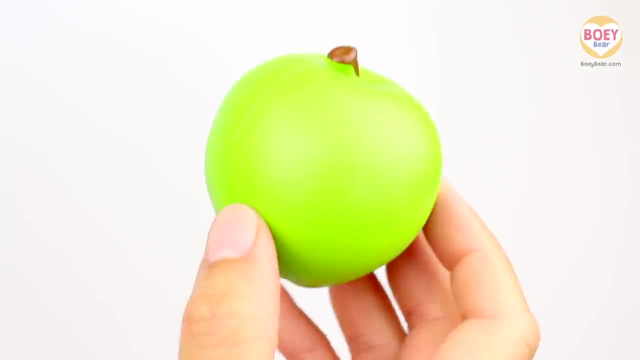 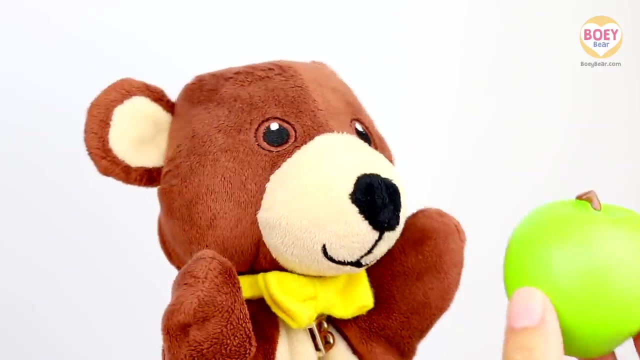 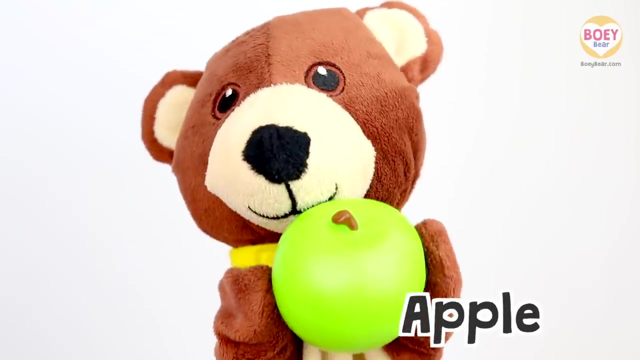 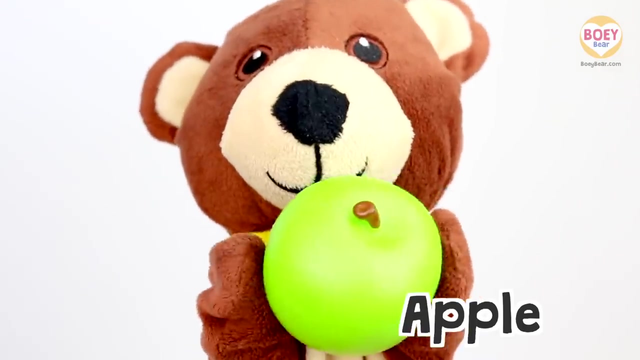 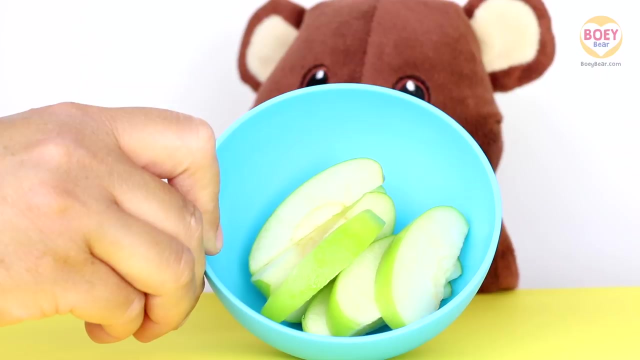 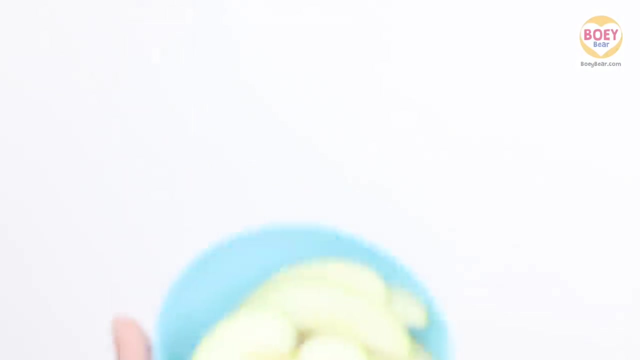 Hmm, it's green and round and grows from a tree. Can you guess what it is? at home It's an apple. Can you say apple, Apple? Well done, Ooh, Here are some apples I've sliced up. Yummy, It's nice and crunchy. 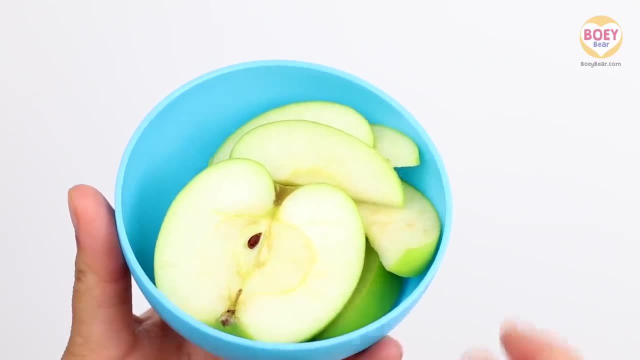 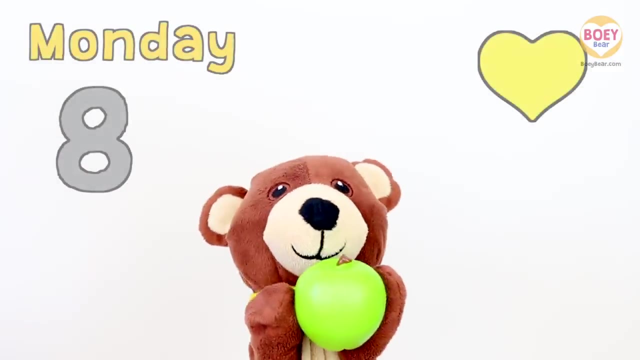 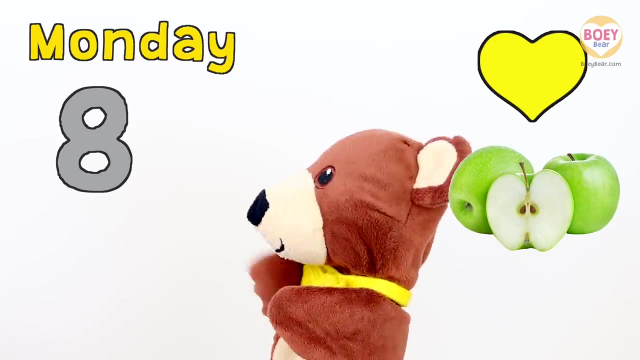 This is the apple core. You can see the seeds. You can see the seed inside. Yum, The fruit of the day is Apple. So let's go over what we've learnt today. Today is Monday. The number of the day is. 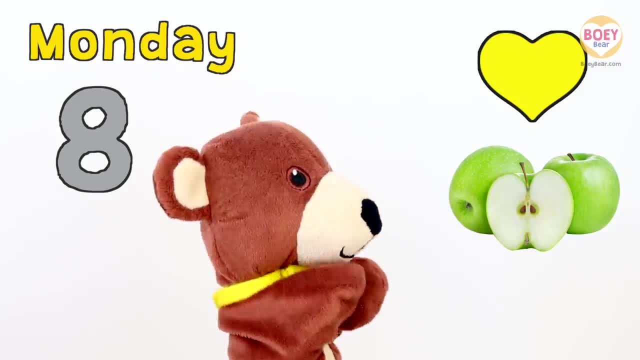 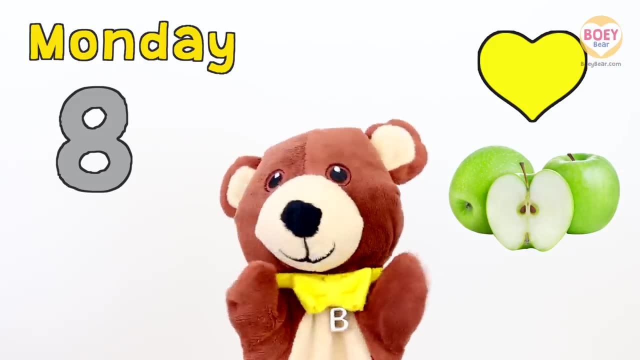 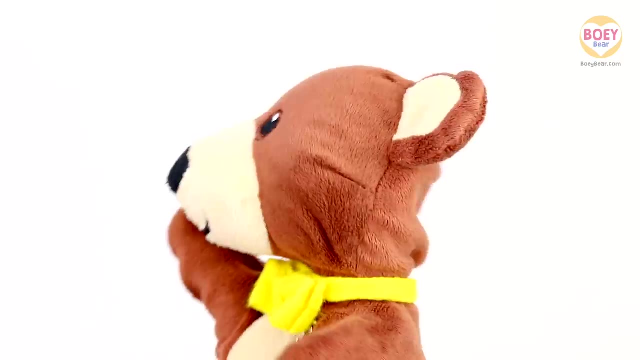 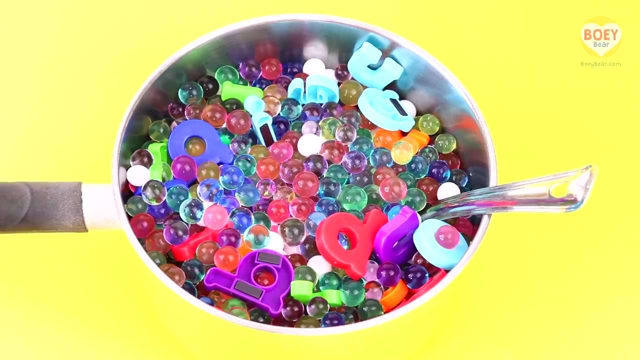 Eight, And today's shape is Heart. And what did we have at snack time? Apple, Apple, Well done. Can you hear that? Ooh, It's time for alphabet soup. Here it is. Oh, wow, It's alphabet soup. 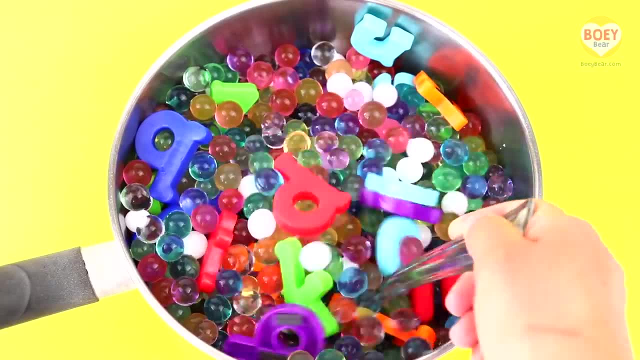 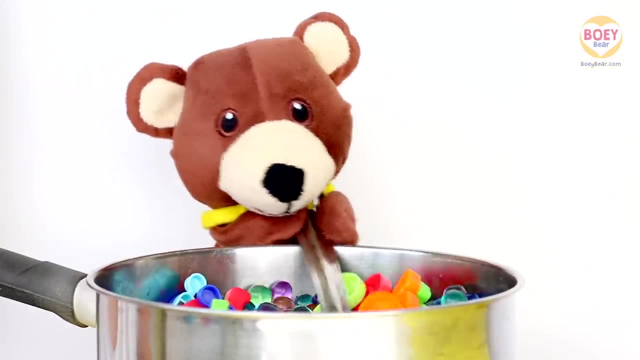 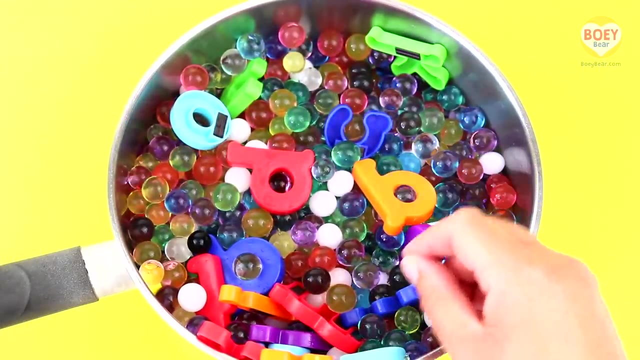 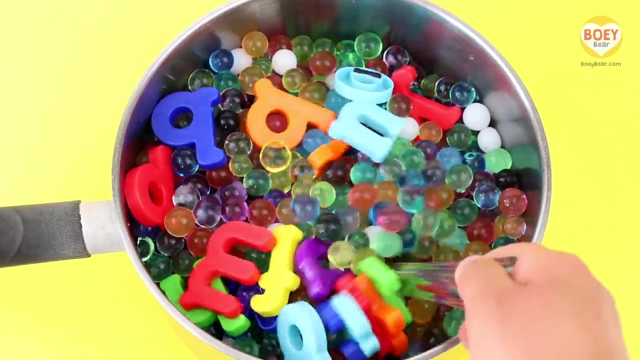 It's a pretend soup, so we can't eat these. It's made up of water, beads and plastic letters. Give it a stir, Bowie, Stir, stir, stir. after Pretend to stir it at home like this. That's it. Let's stir it together. Here's. 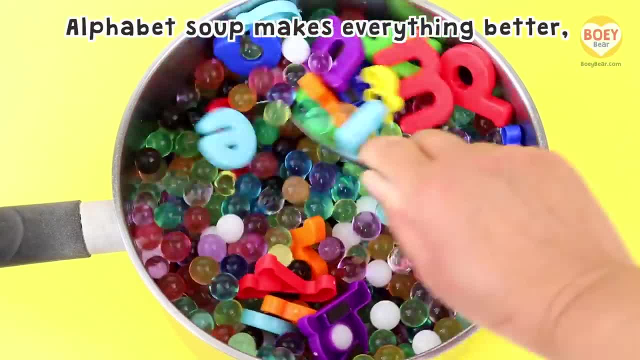 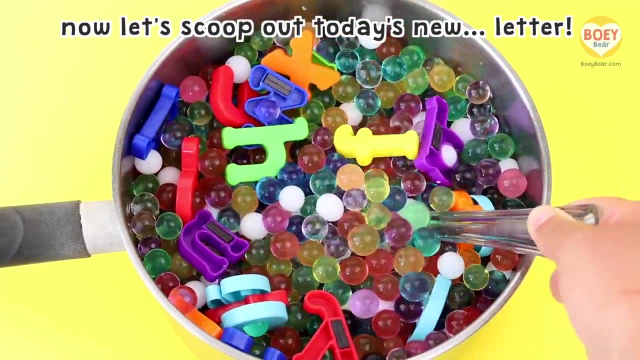 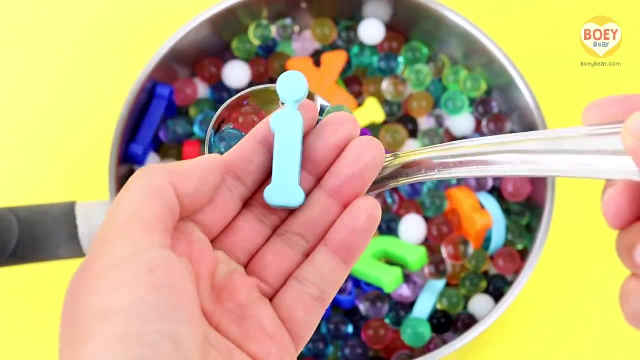 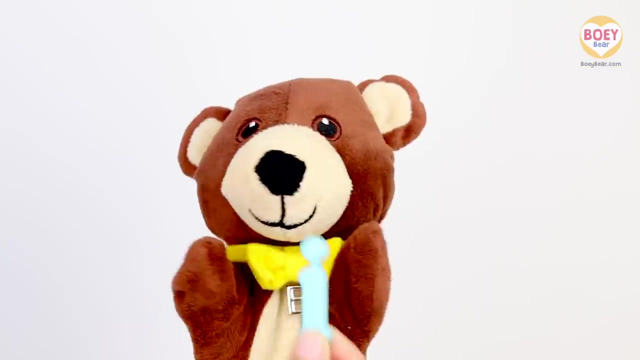 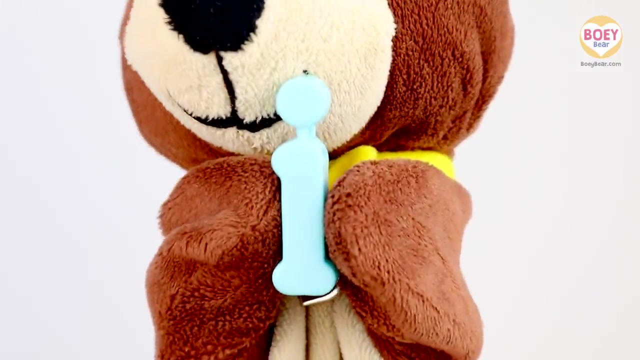 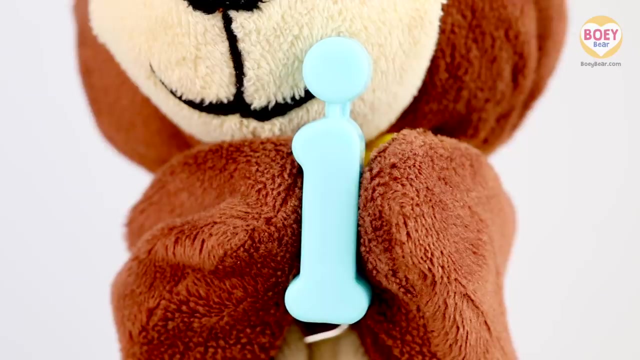 our special rhyme: Alphabet: soup makes everything better. Now let's scoop out today's new letter. Can you see what letter it is? It's the letter I, And the sound it makes is I. Here you go, Bowie, Thank you, I, I, I. Now it's your turn at home. Can you say: I, I, I. Well done. 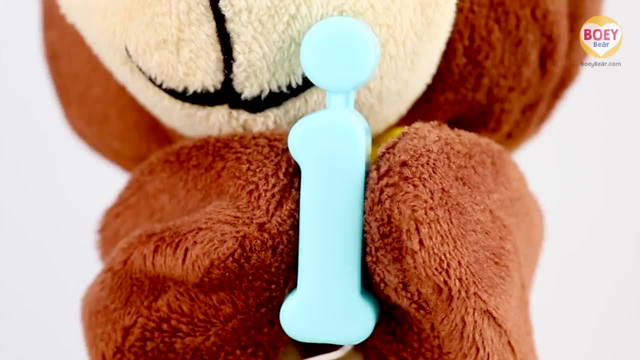 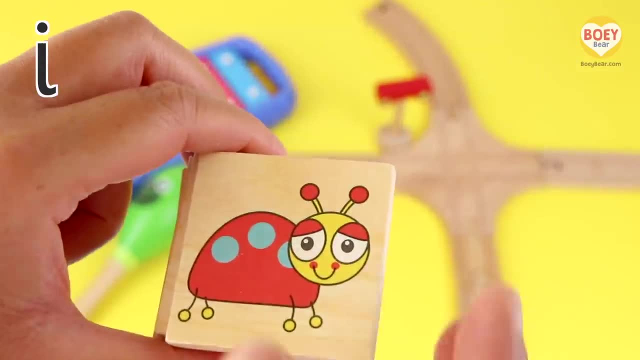 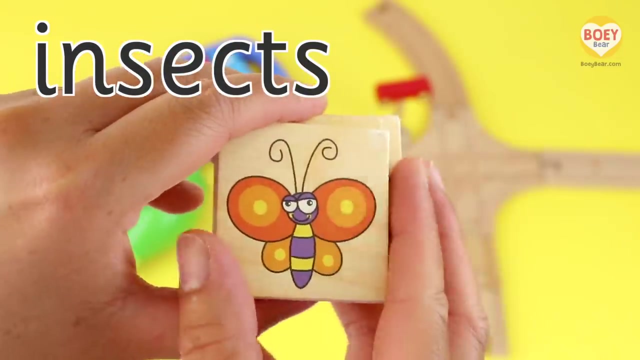 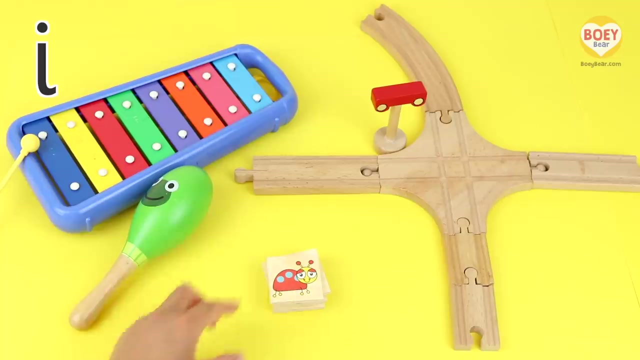 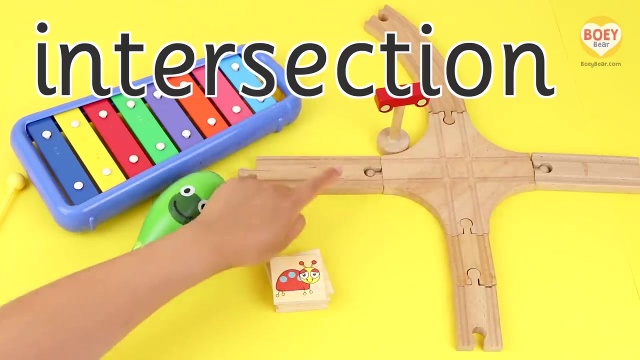 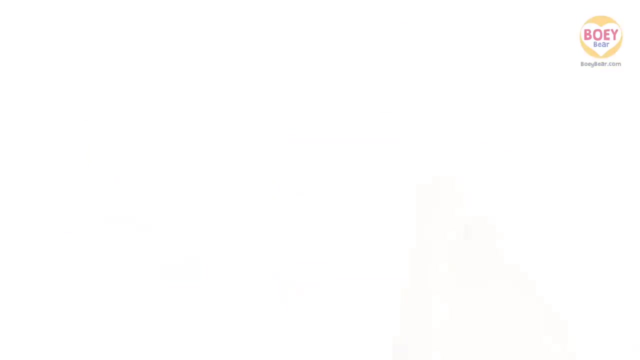 What things begin with the letter I. Let's see, These are I I insects, Insects. Here we have insects. I I instruments- Instruments to make music. This is an I? I intersection, Intersection Where roads or tracks meet. Now let's learn how to write the letter. Get your finger up. 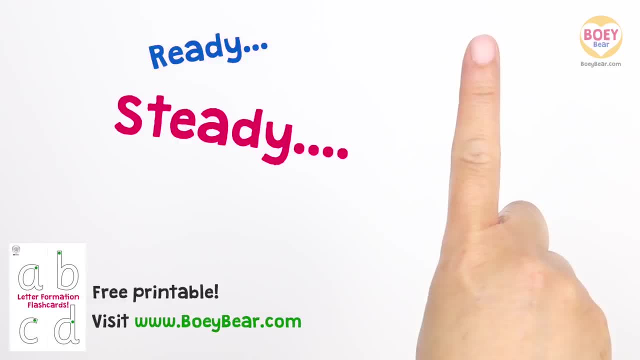 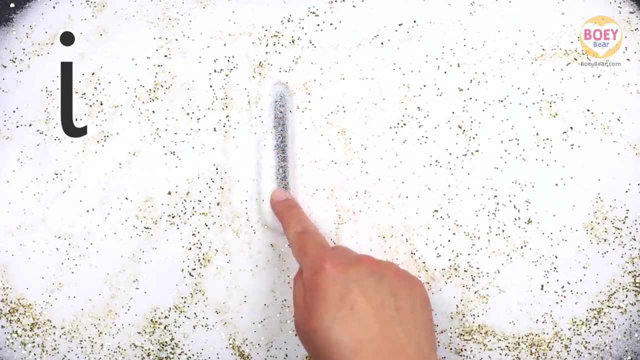 in the air and copy along: Ready, steady, go, Start at the top, Go straight down and give a little flick And a dot at the top. Let's do it again, but a bit faster. Copy along with your finger in the air. Well done So. 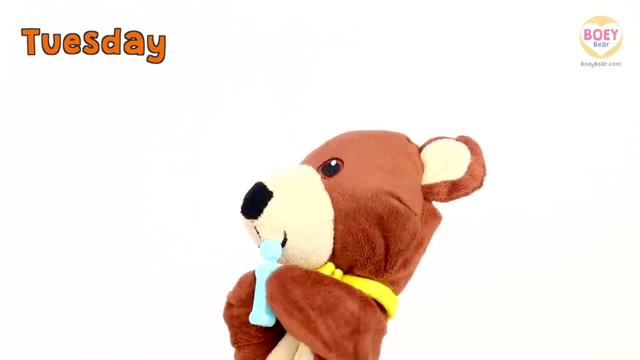 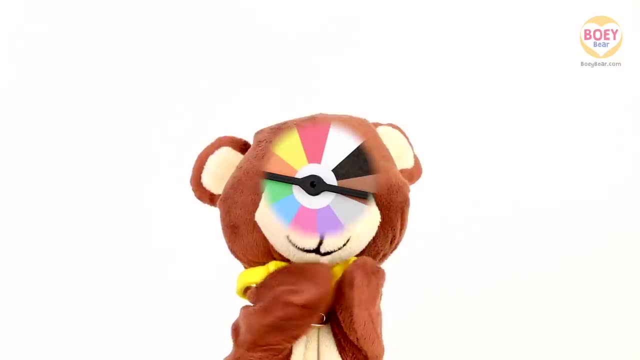 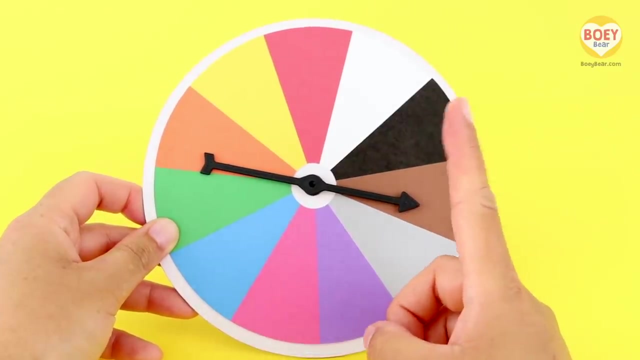 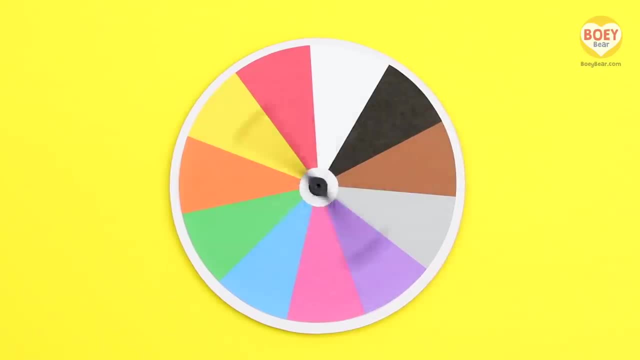 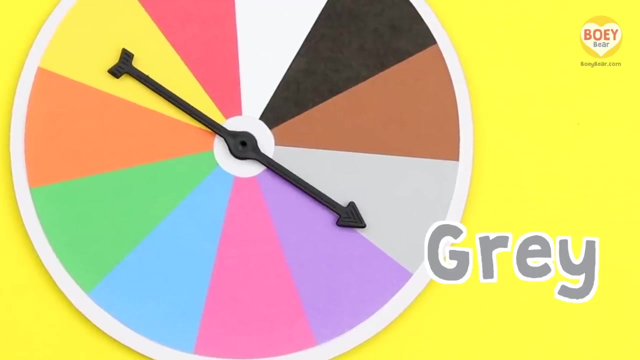 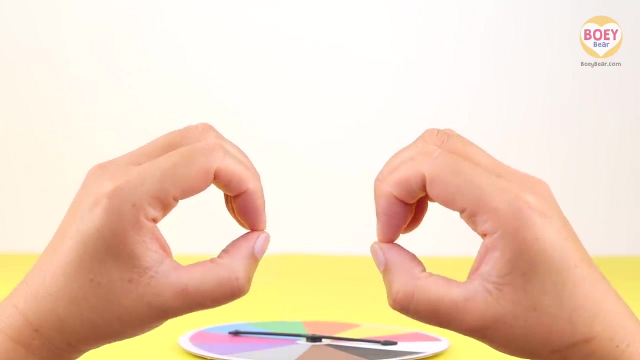 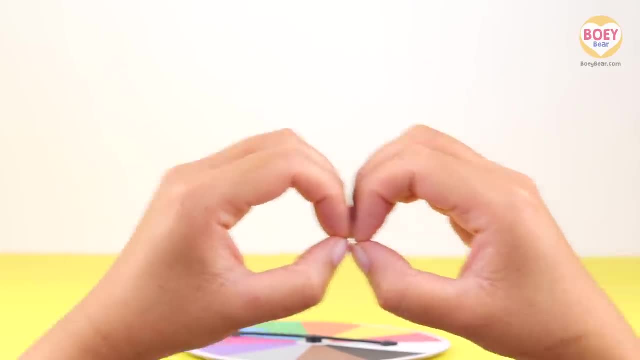 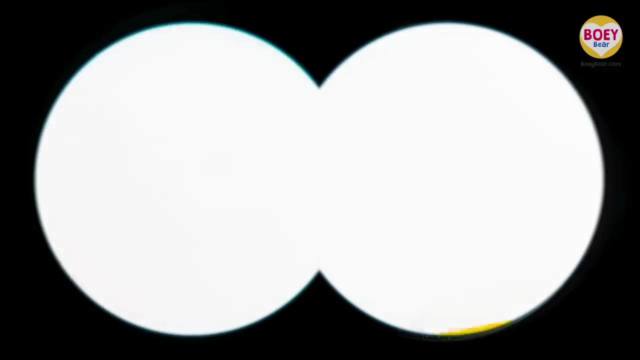 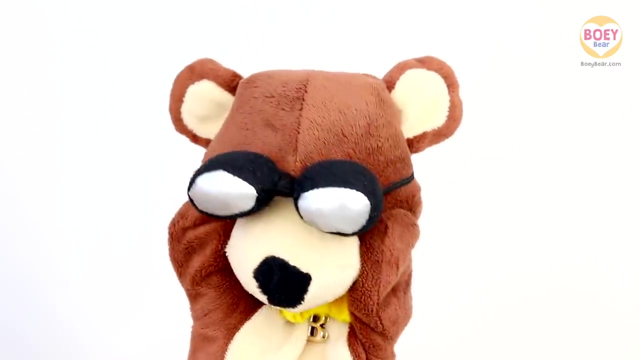 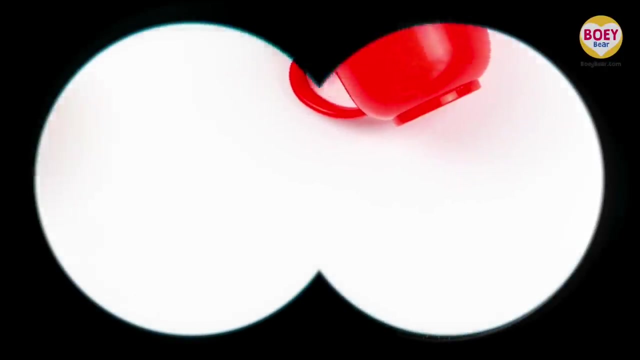 From where you are sitting, can you see something that is grey? Parece colourful com colored eyes. Have a look for today's colour. What did you find at home? Hmm, what can we see that is grey? Oh, what was that? 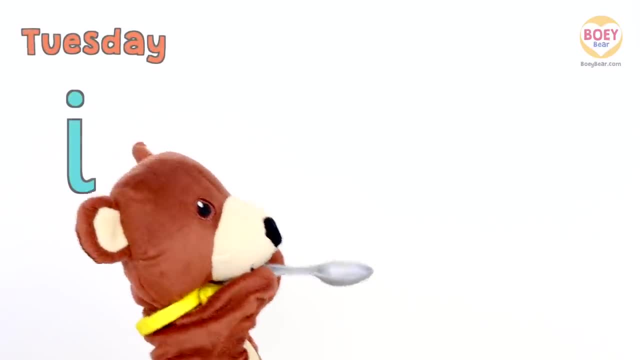 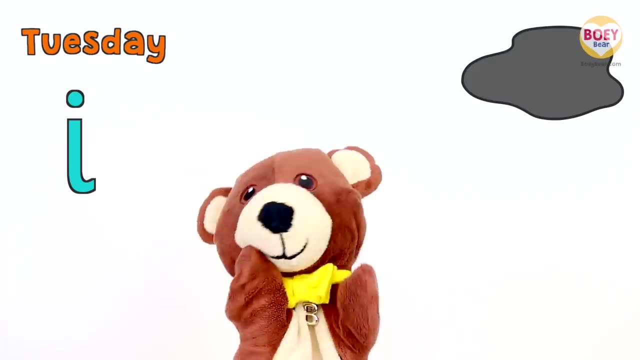 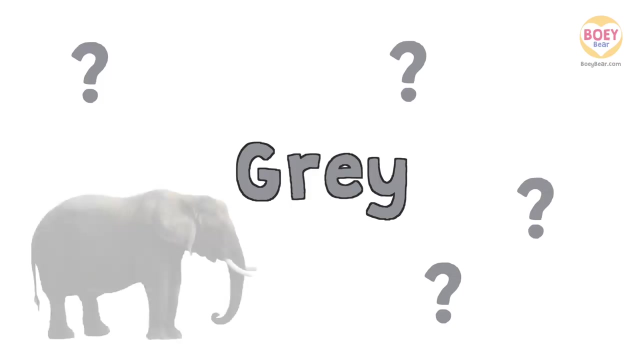 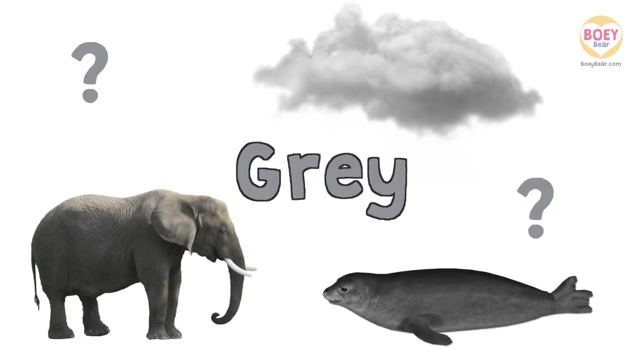 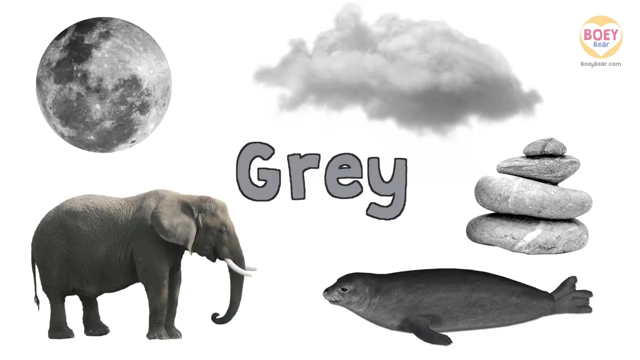 It's a grey spoon, So the colour of the day is grey. What other things around us are grey? Get ready to answer. A grey Elephant And a grey Cloud, A grey Moon Seal, A grey Moon, Grey Stones. Well done, Was that your tummy rumbling Bowie? 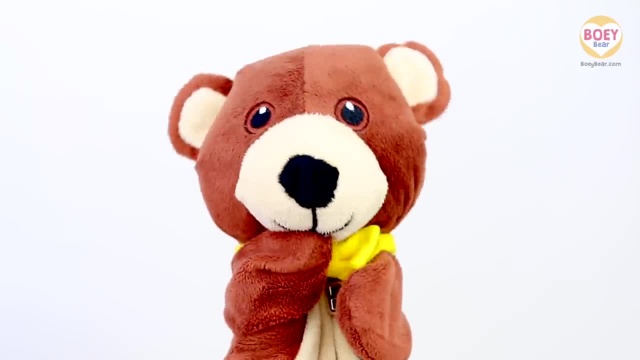 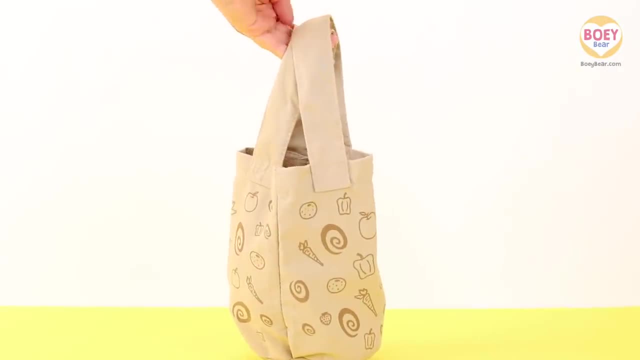 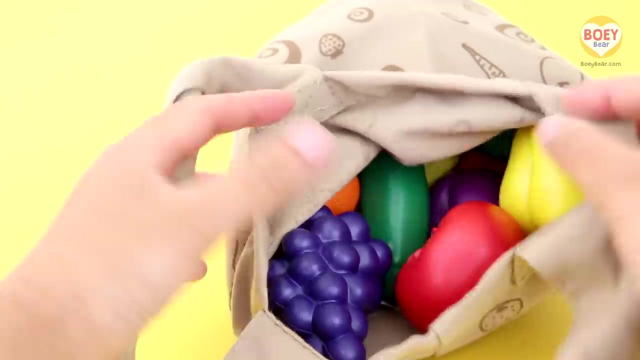 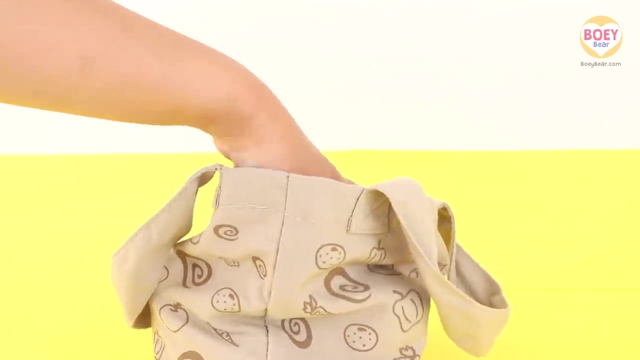 Was it your tummy at home? Oh, it might have been mine. I think we're all. I think we're all hungry. It must be snack time. Here's my grocery bag. It's full of different fruits and vegetables. Have a look, I'm going to put my hand in and pick out a fruit or vegetable for today. 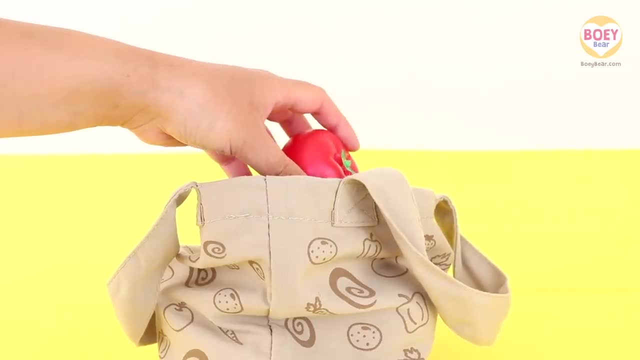 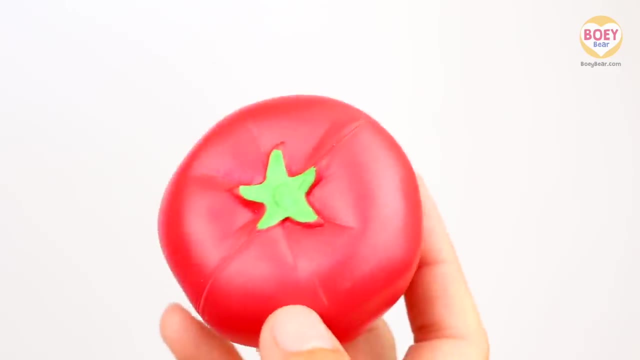 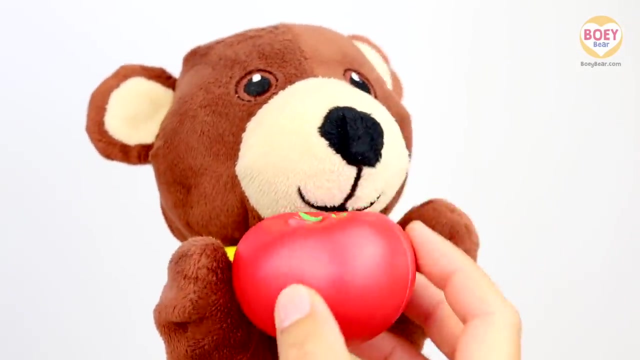 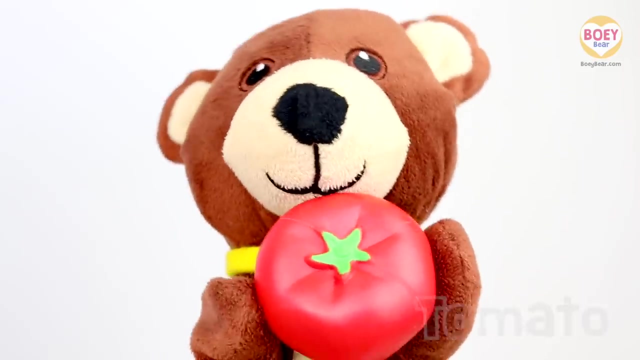 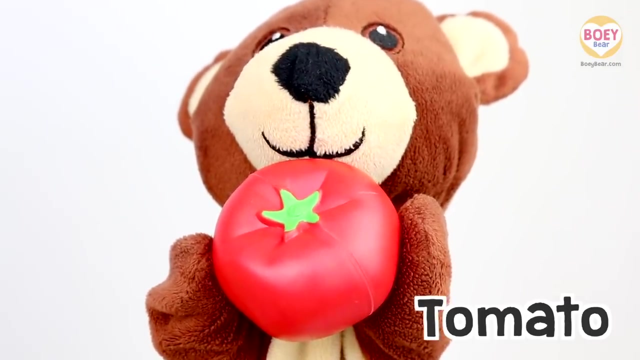 You have to guess what it is. Hmm, it's red, It has skin on the outside and a little bit of skin on the inside, And it's juicy inside. Thank you, What do you think it is? It's a tomato. Can you say Tomato? Well done. 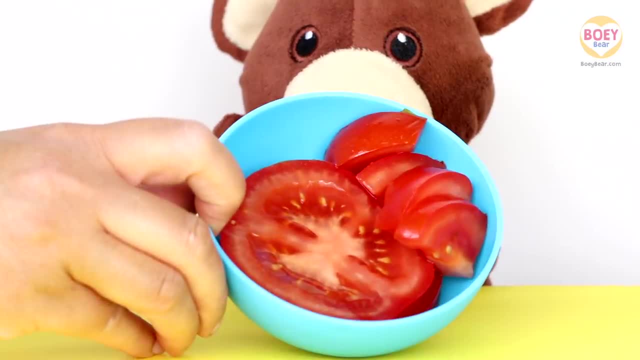 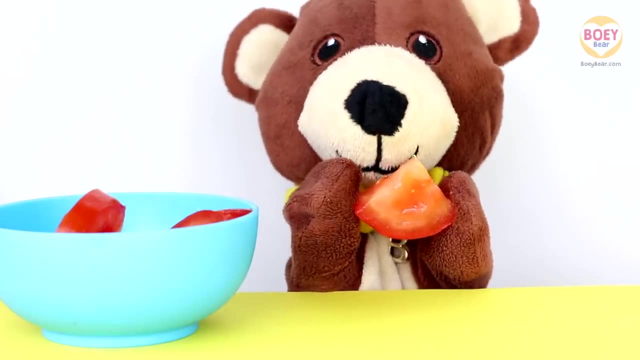 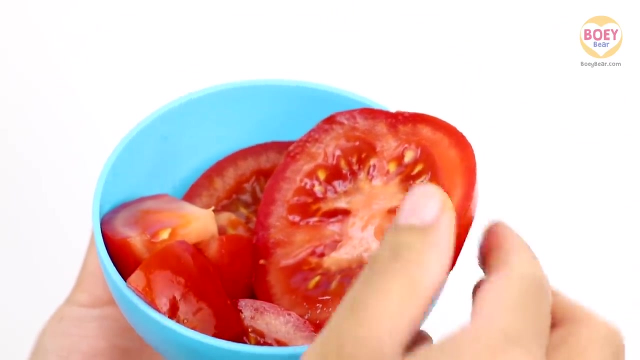 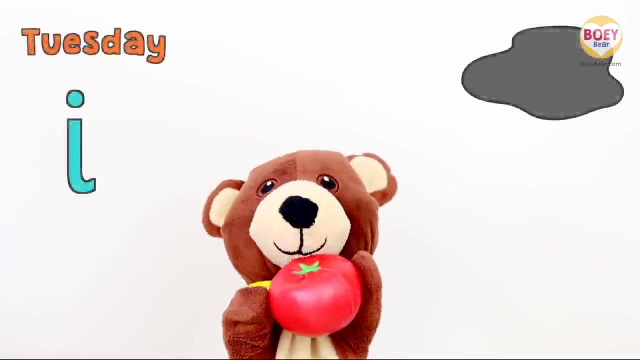 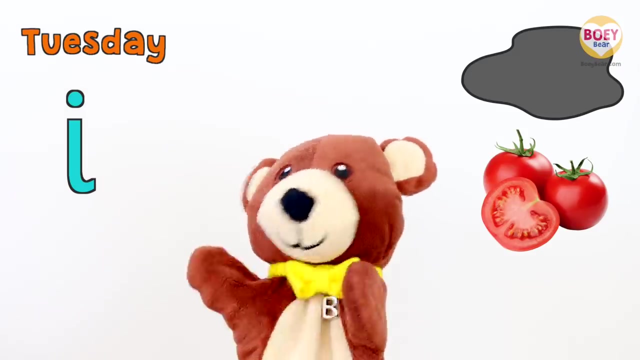 Here's some tomato that I've cut up for us to eat. Well done, Mmm. tasty, Yummy. It's sweet and juicy And it has little seeds inside that you can eat. Yum. So we have a Tomato. So let's go over what we've learnt today. 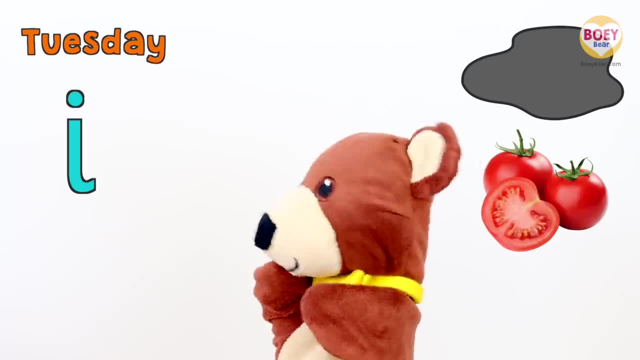 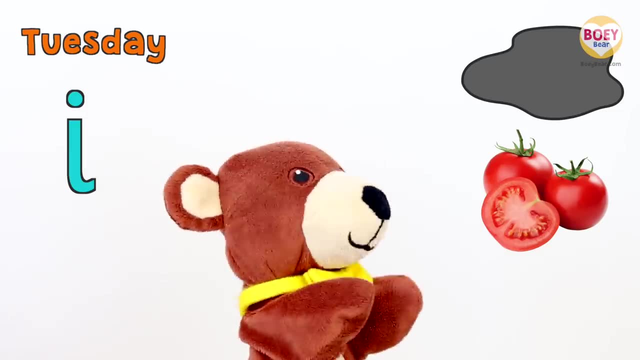 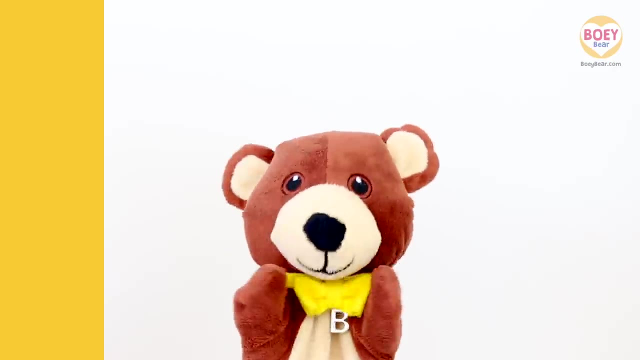 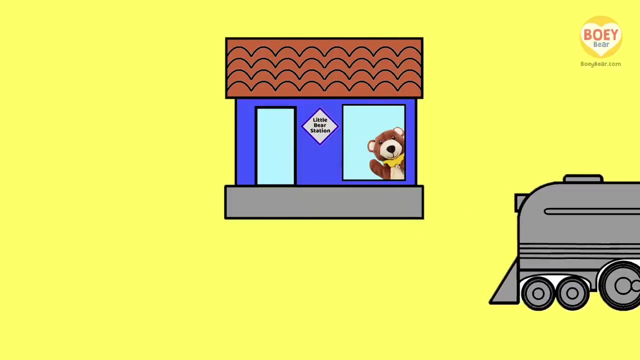 Today is Tuesday, The letter of the day is I And today's colour is Grey. And what did we have at snack time? Tomato, Well done. Can you hear that A train? Ooh, It's the number train. Let's see what number stops at the station today. 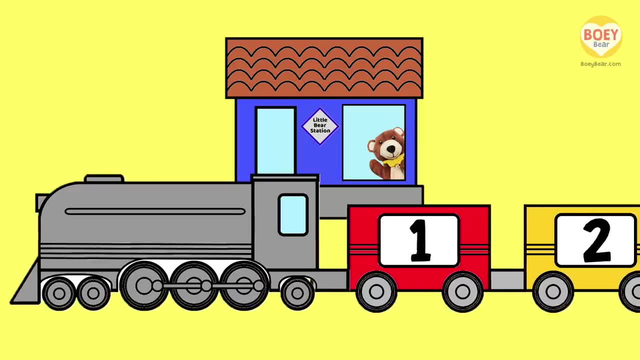 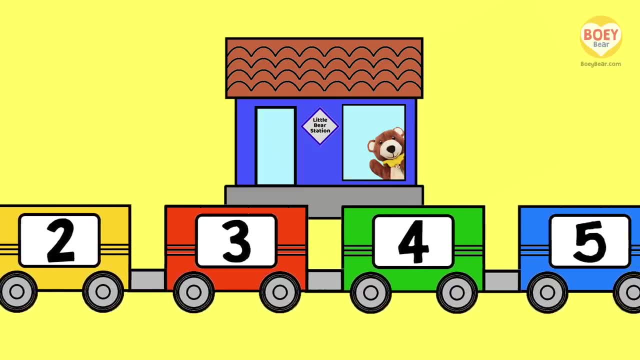 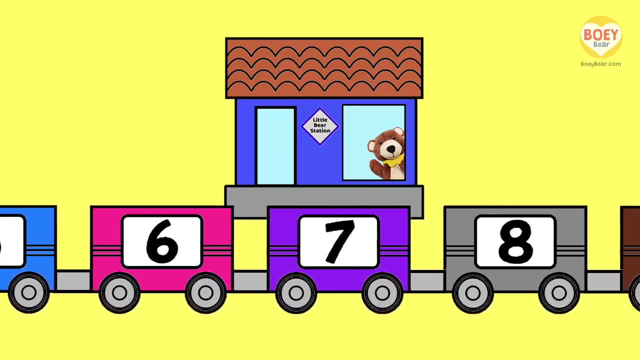 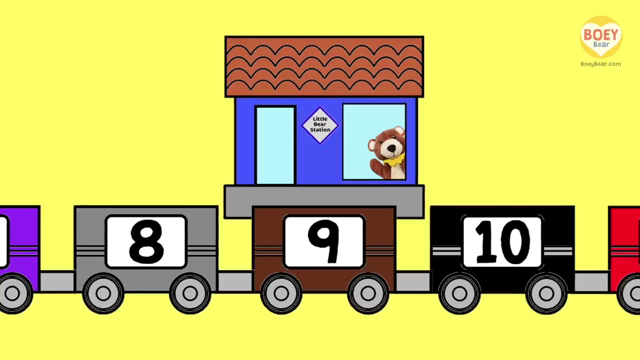 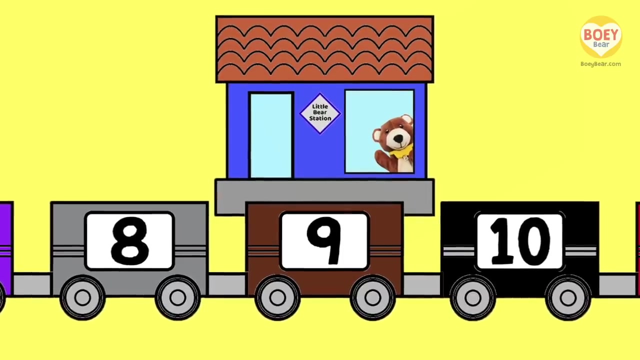 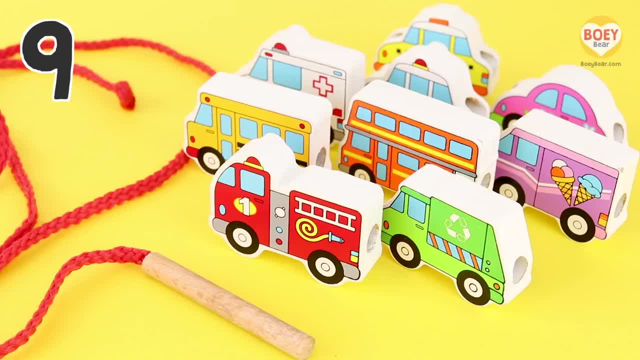 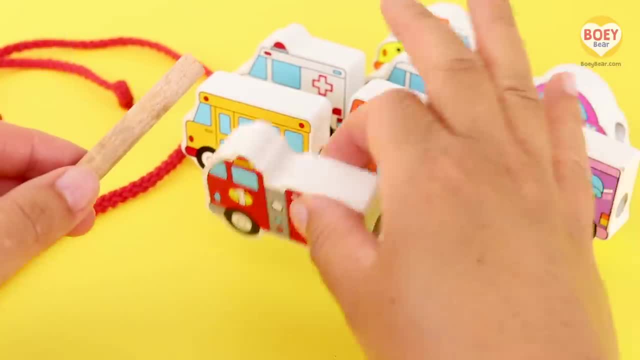 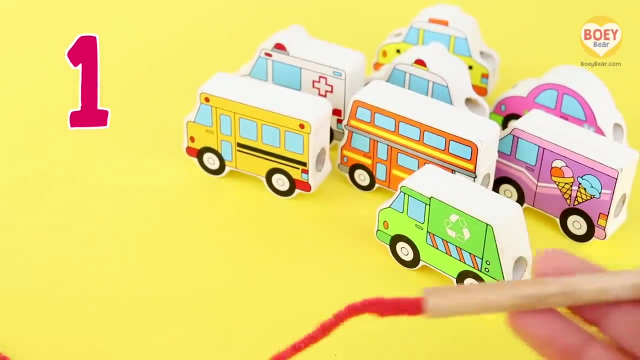 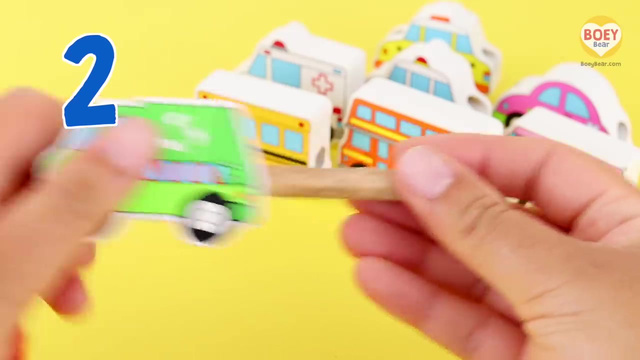 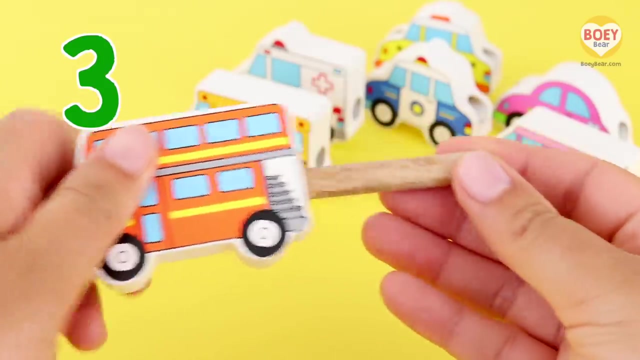 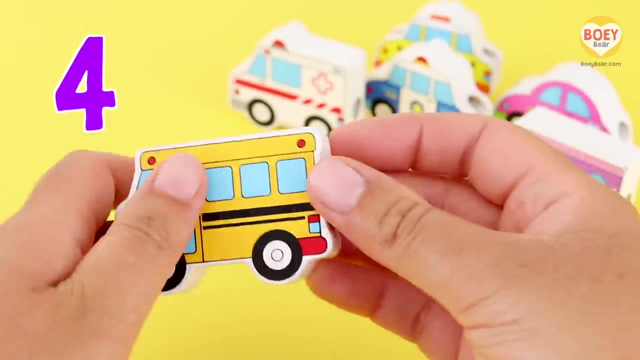 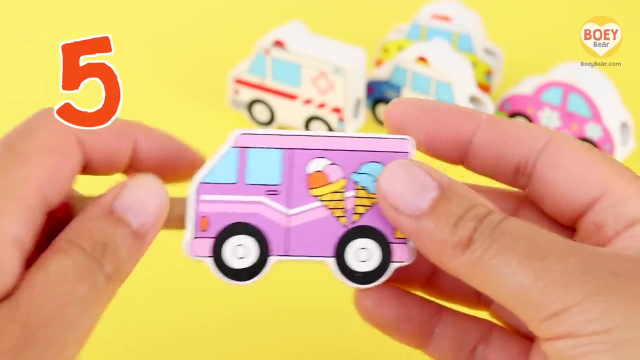 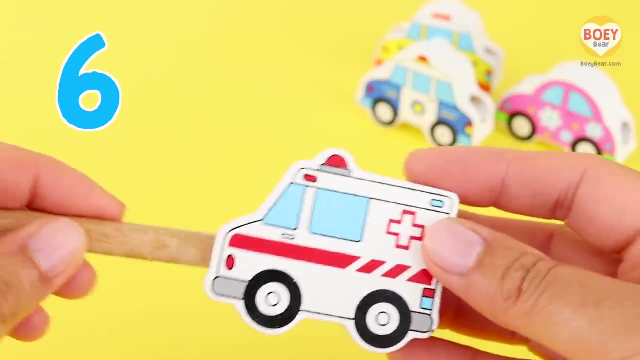 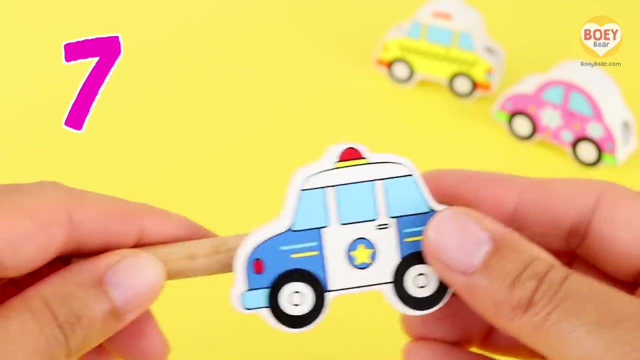 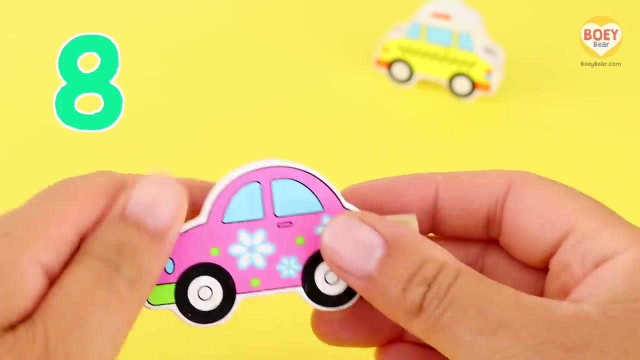 Now let's count the number. We should have nine vehicles here To thread onto this rope. Let's count them: One, Two, Three, Four, Five, Six, Six, Seven, Eight, Nine, Ten, Eleven, Twelve, Thirteen, Thirteen, Thirteen, Four, Four, Five, Four, Four, Five, Six, Seven, Eight, Nine, Nine. 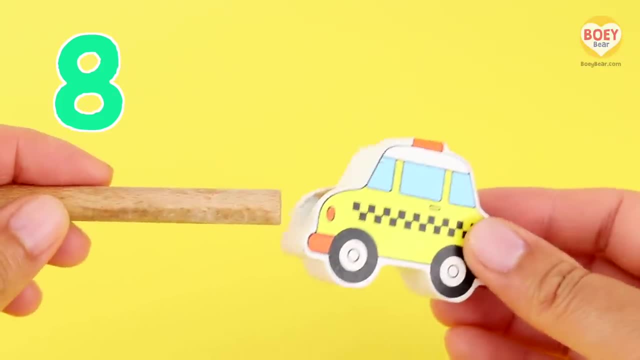 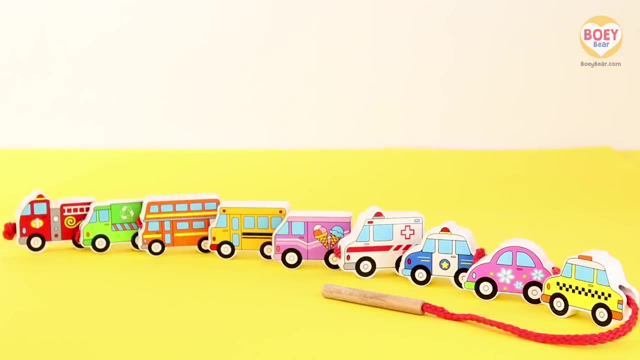 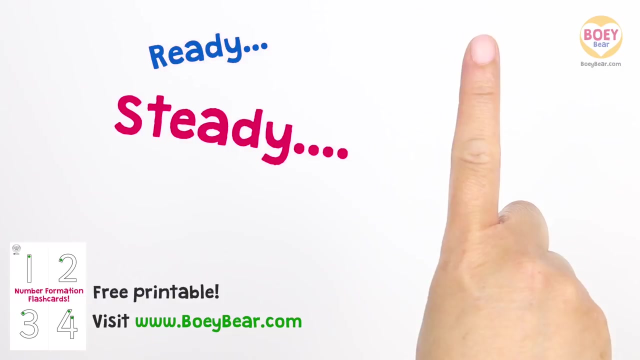 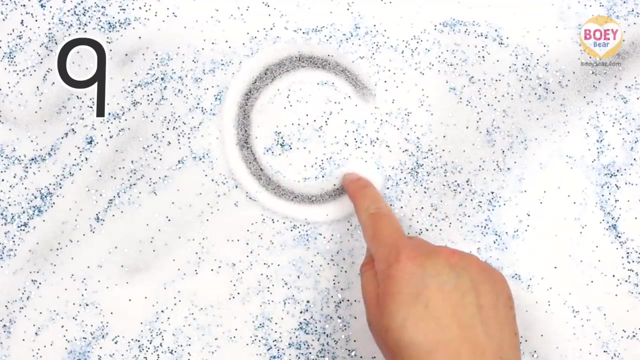 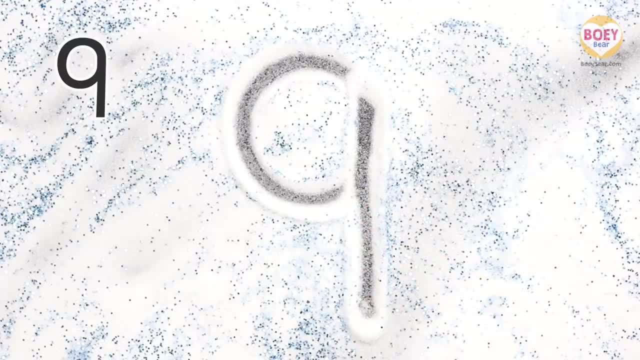 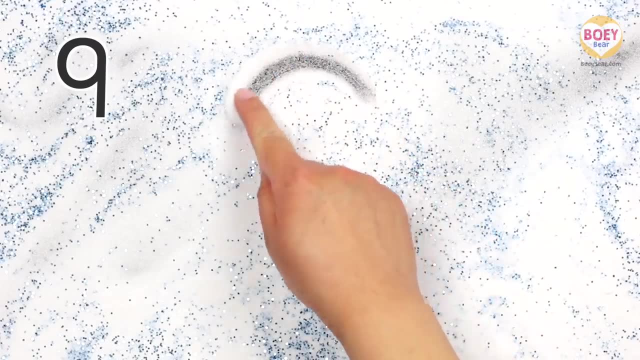 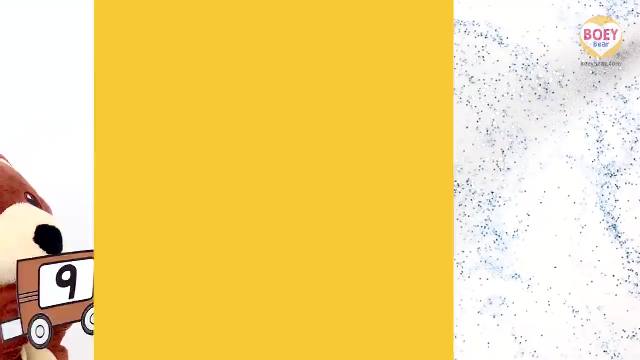 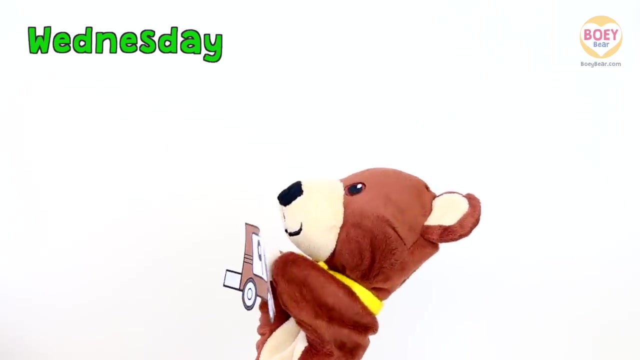 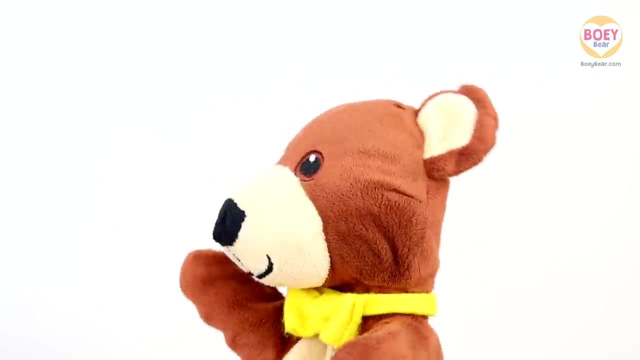 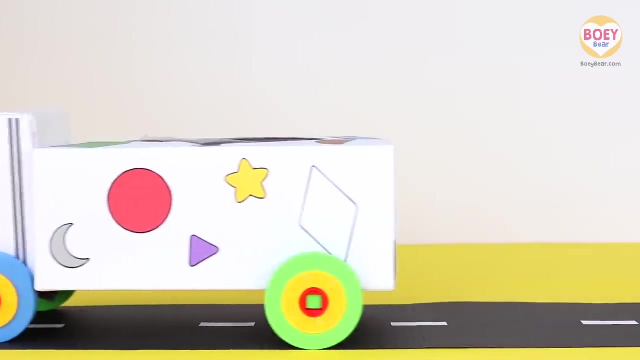 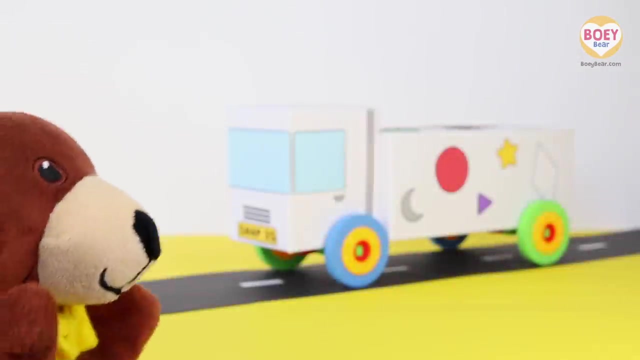 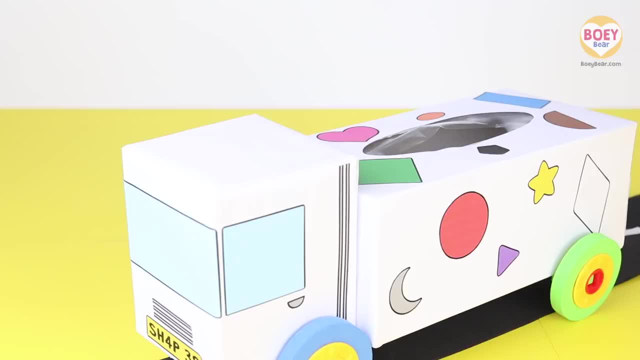 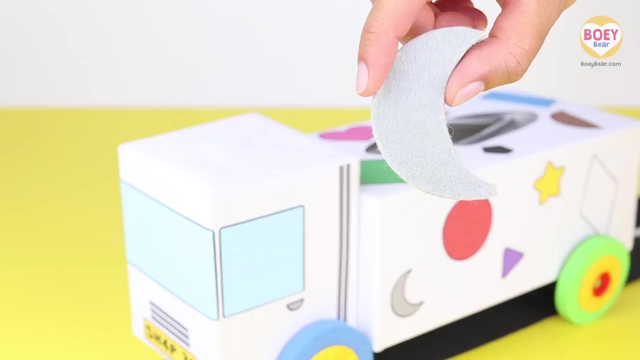 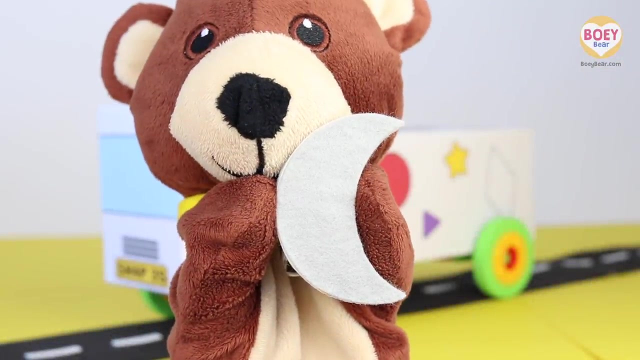 i'm going to put my hand in and see what shape we have today. hmm, it has two curves and two points. can you guess what shape it is? it's a, b, Crescent. Can you say crescent Crescent? Well done, It has two curves, one, two, and two points. one two. 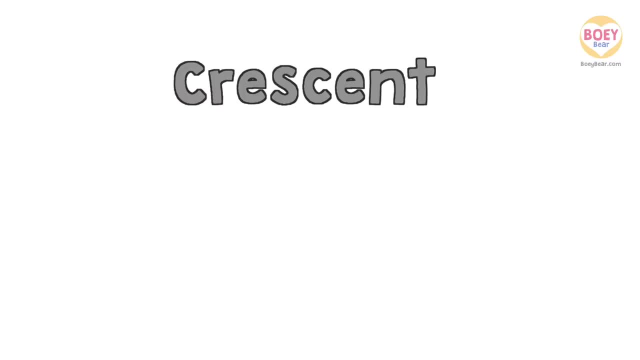 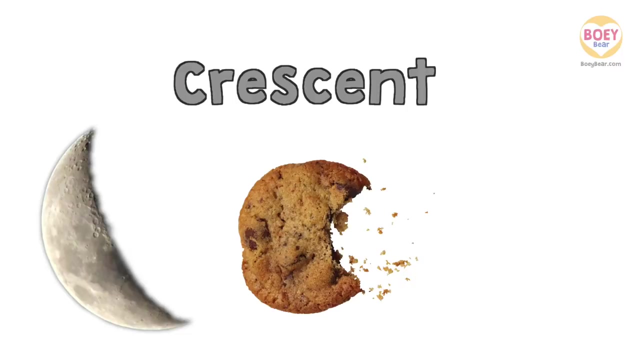 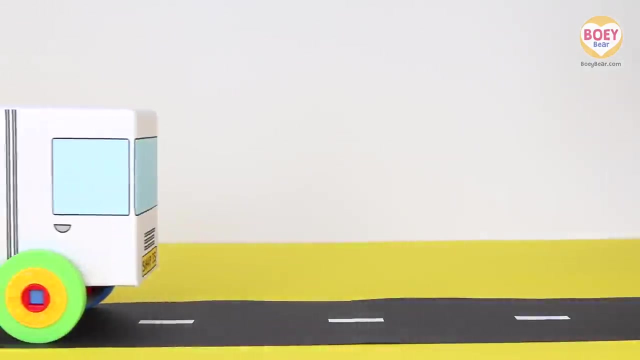 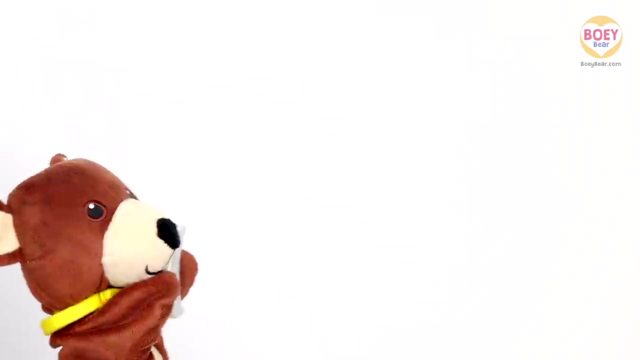 What things around us are crescent-shaped. Get ready to answer: A crescent-shaped moon, a crescent-shaped cookie and a crescent-shaped banana- Great, Thank you, Shapes Truck. So today's shape is a crescent And today's shape is a crescent. 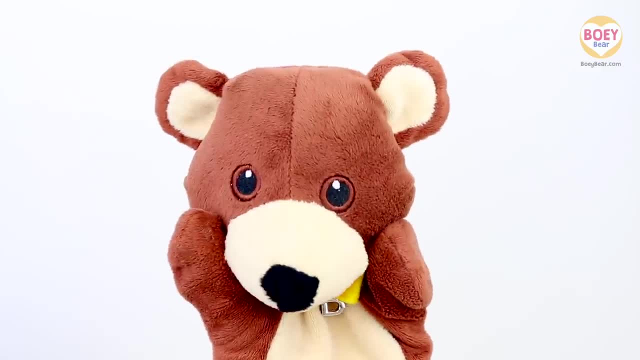 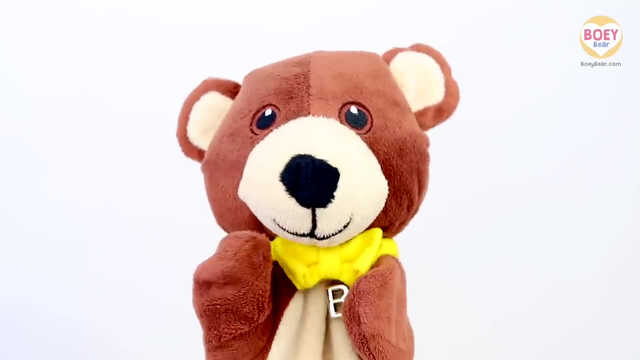 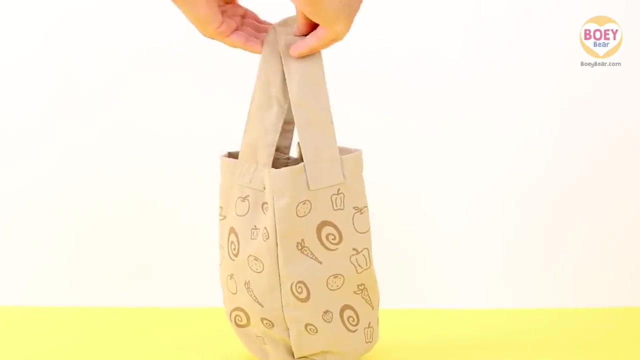 Yay, Was that your tummy rumbling Bowie? Was it your tummy at home? Oh, it might have been mine. I think we're all hungry. It must be snack time. Here's my grocery bag. It's full of different fruits and vegetables. 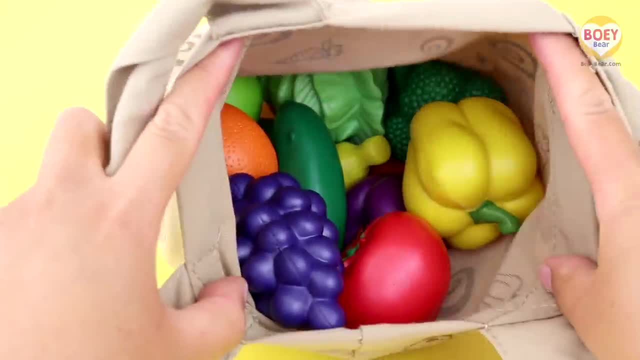 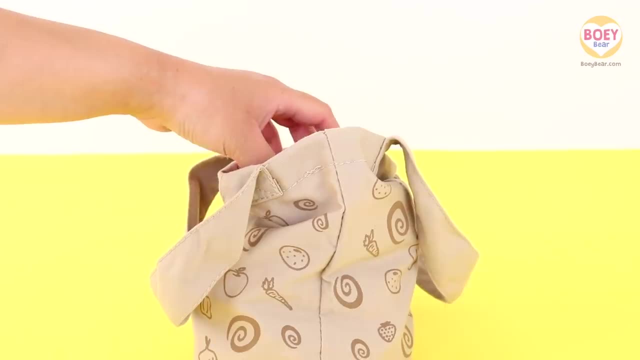 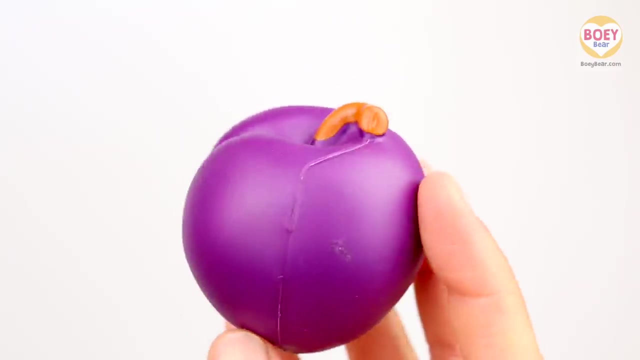 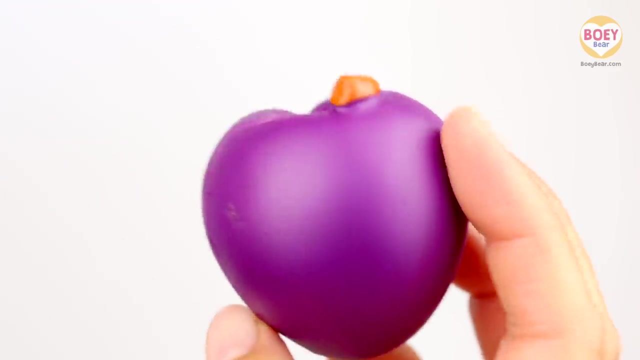 Have a look. I'm going to put my hand in and pick out a fruit or vegetable for today. You have to guess what it is. It's a fruit. It's purple and round, It has skin on the outside And it's juicy inside. 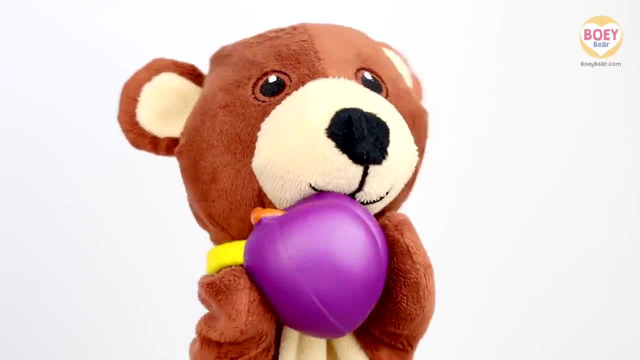 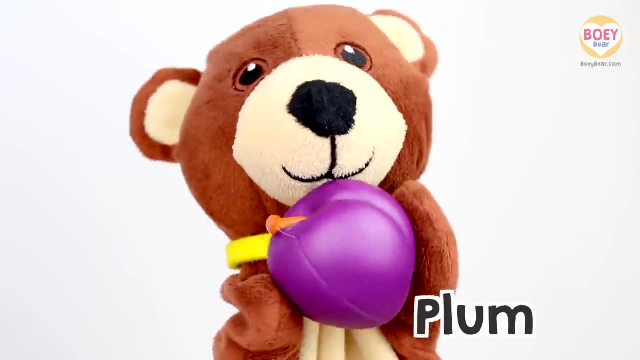 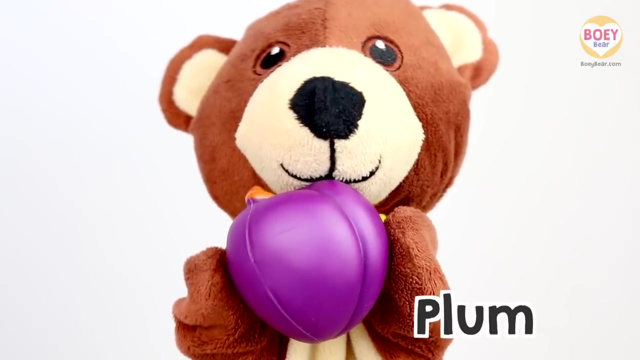 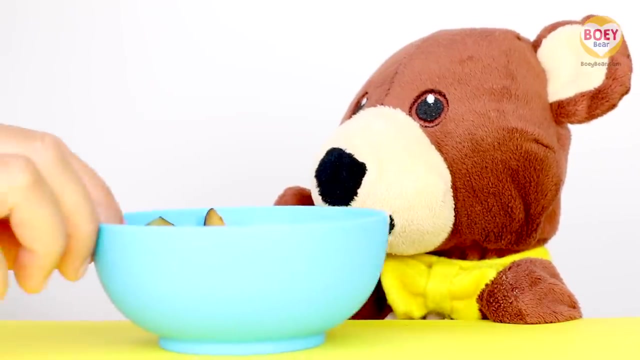 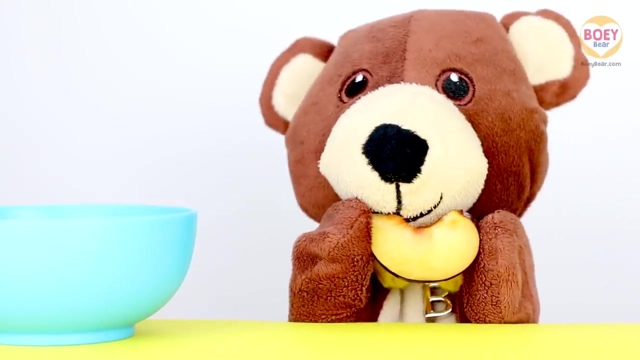 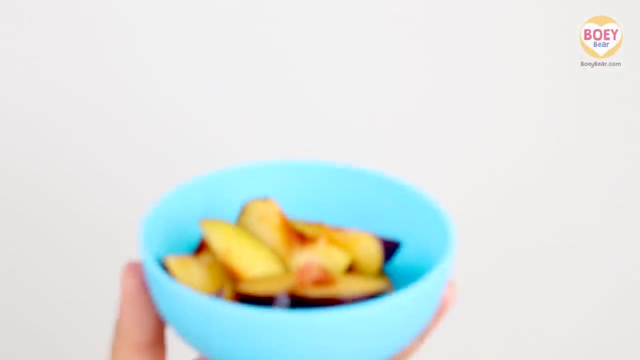 Here you go, Bowie, Thank you. Can you guess what it is? At home It's a plum. Can you say plum, Plum, Great Ooh, It's nice and sweet. Yummy, I'm going to have a plum too. 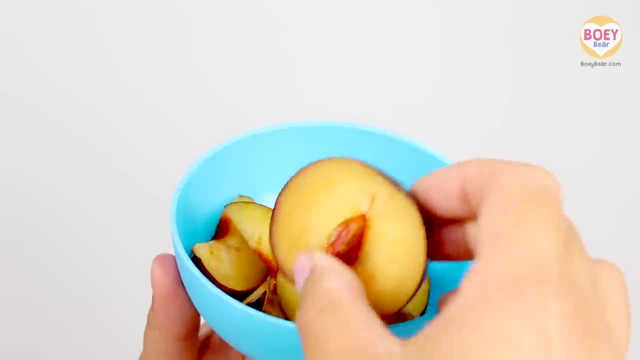 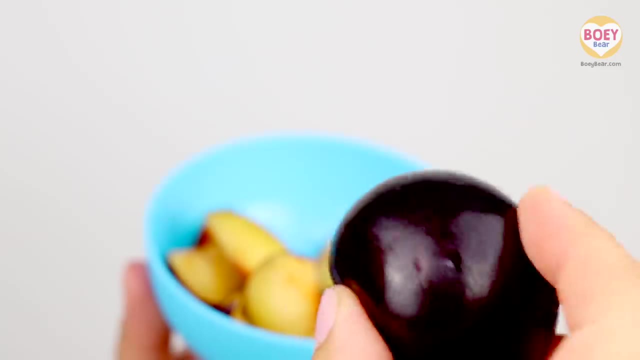 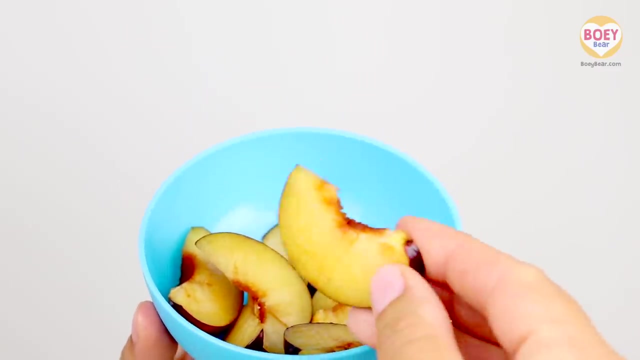 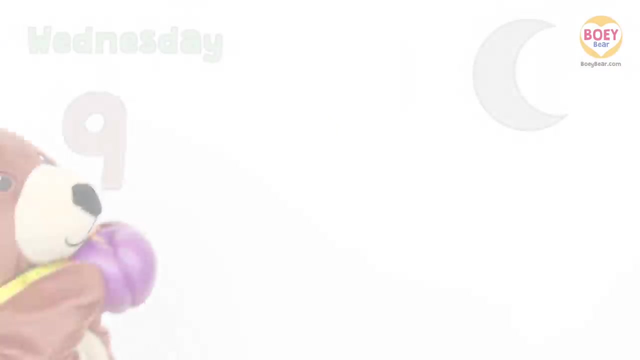 Here's half a plum And you can see the stone inside that you can't eat. You just eat around it. Yum, Here are some plum slices. It's sweet and juicy. The fruit of the day is: I'm going to have a plum. 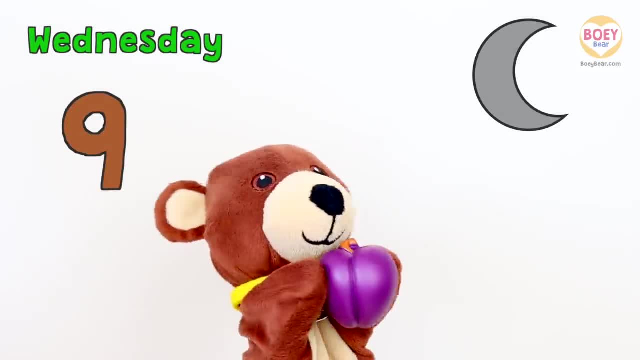 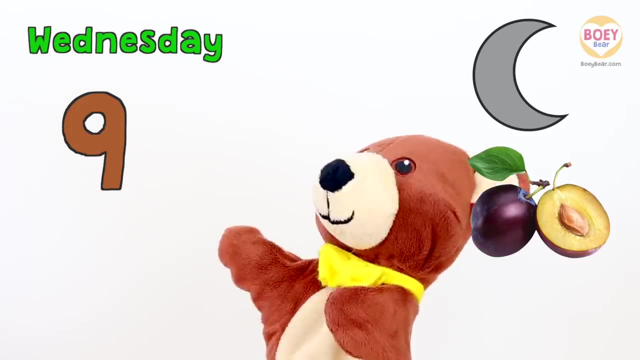 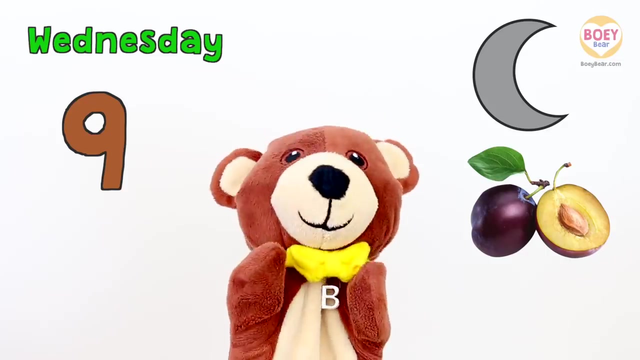 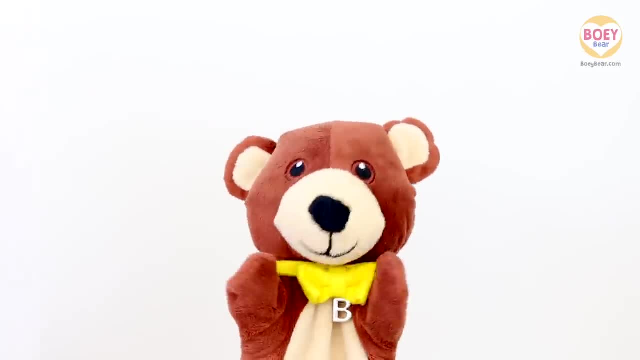 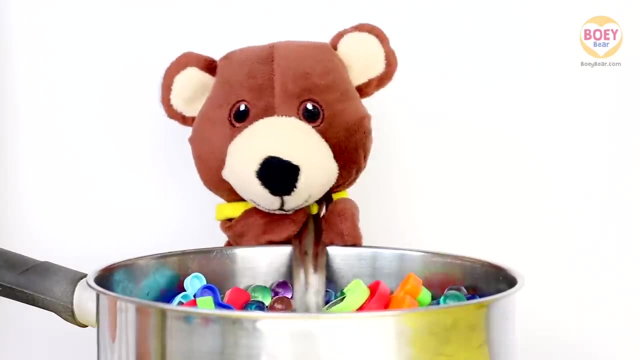 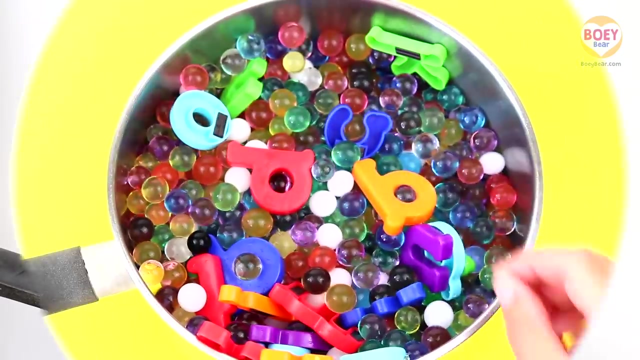 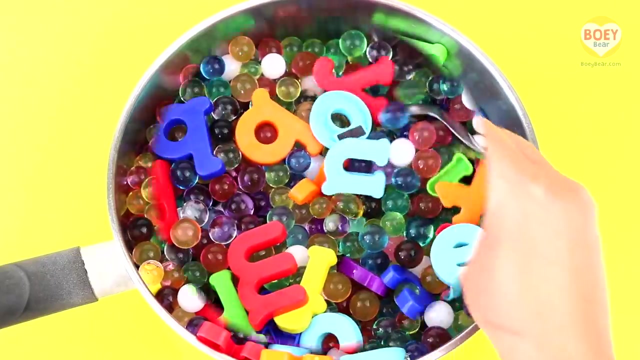 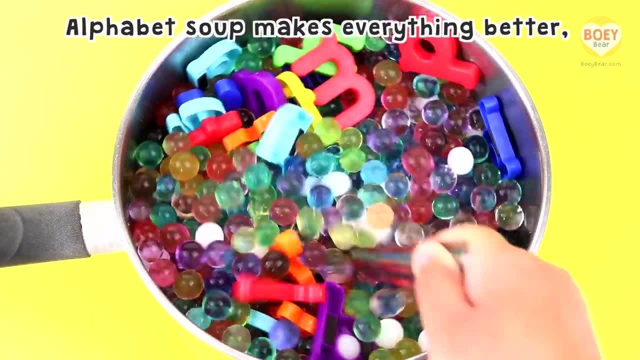 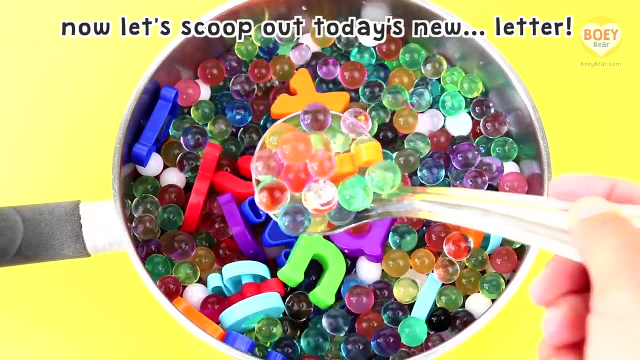 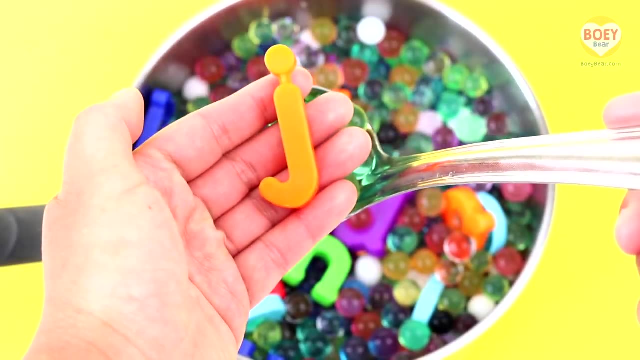 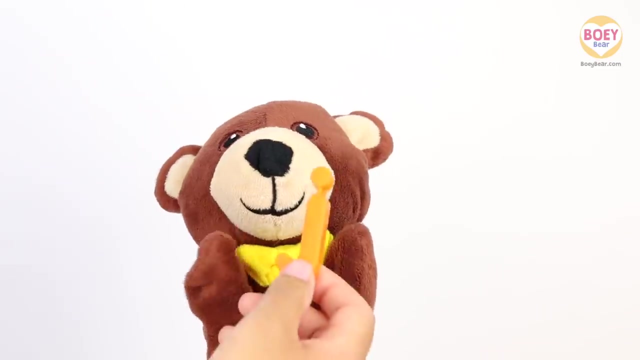 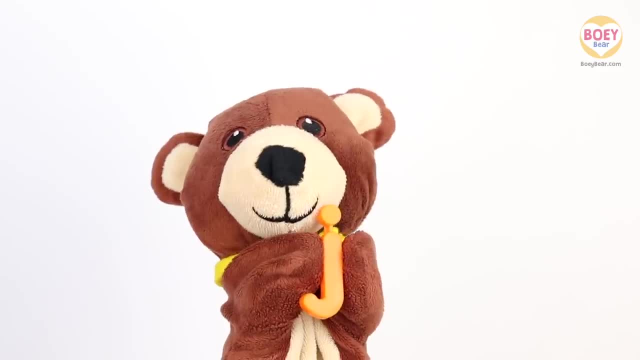 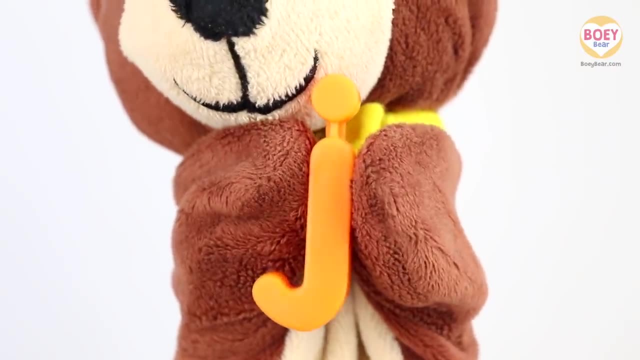 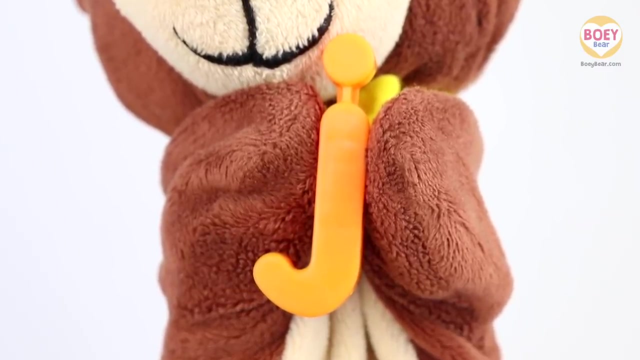 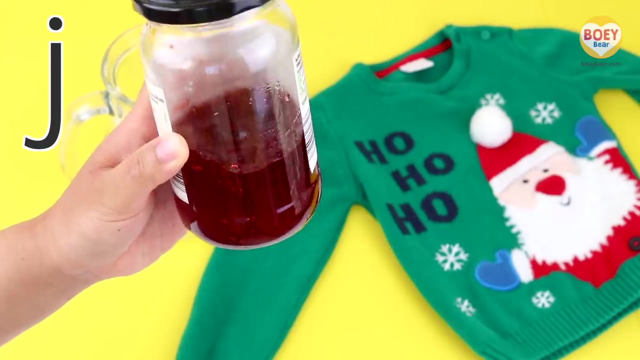 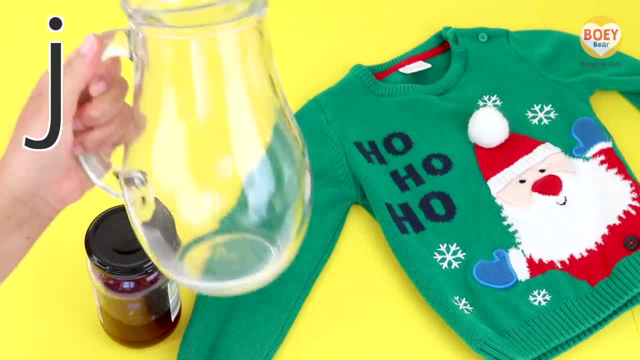 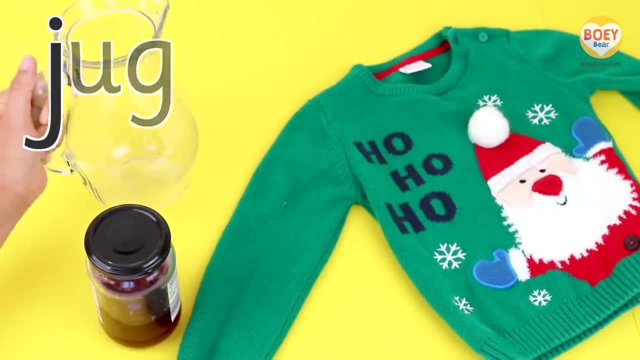 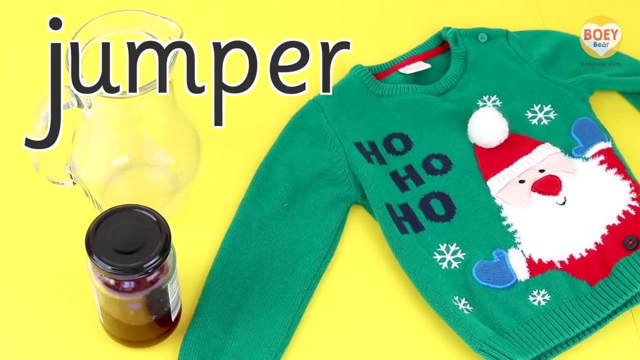 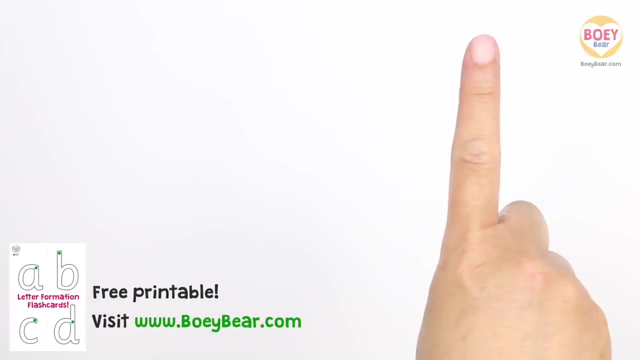 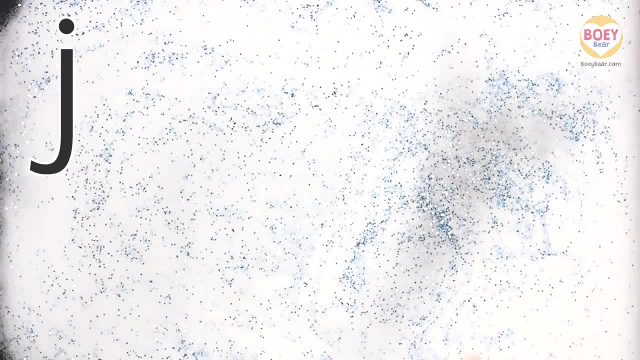 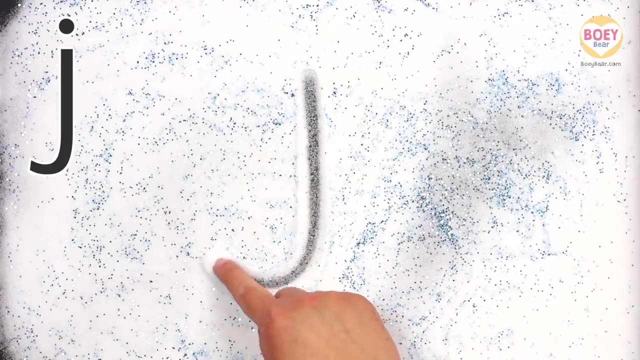 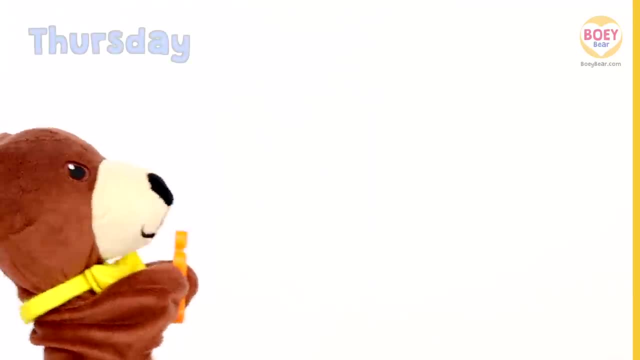 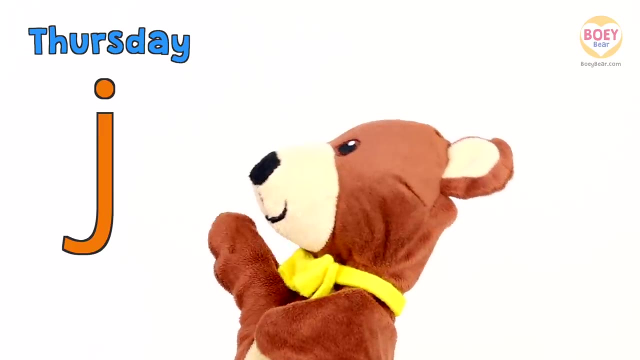 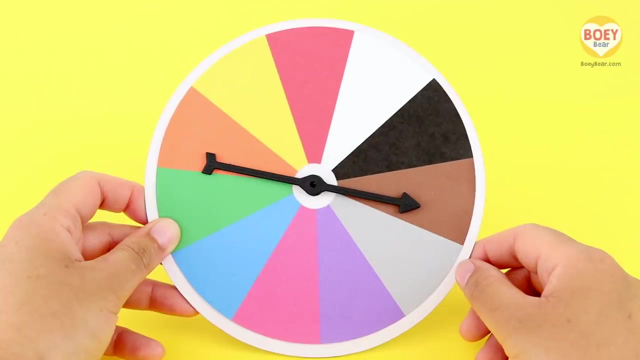 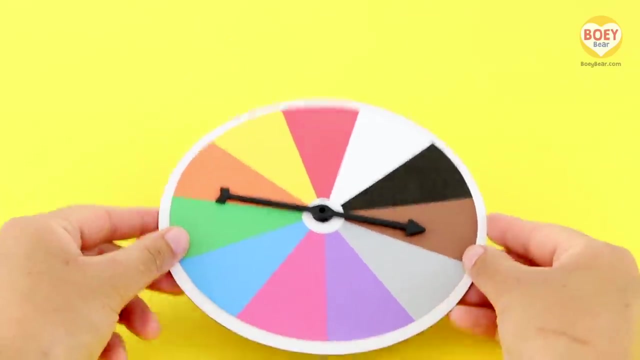 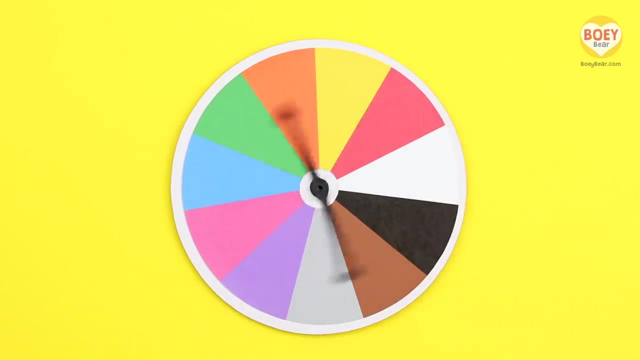 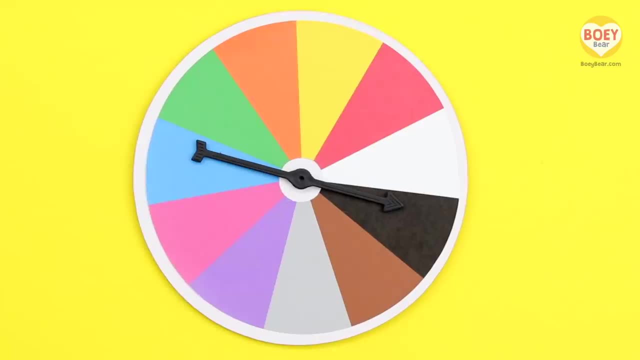 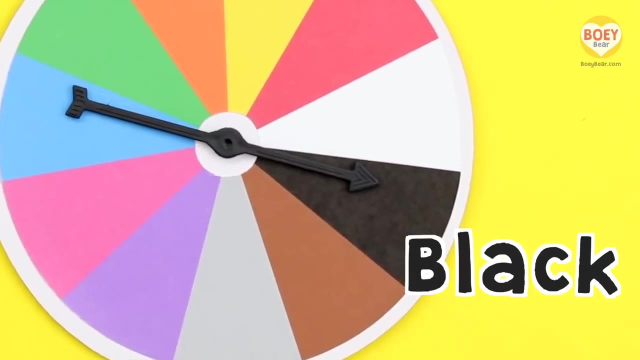 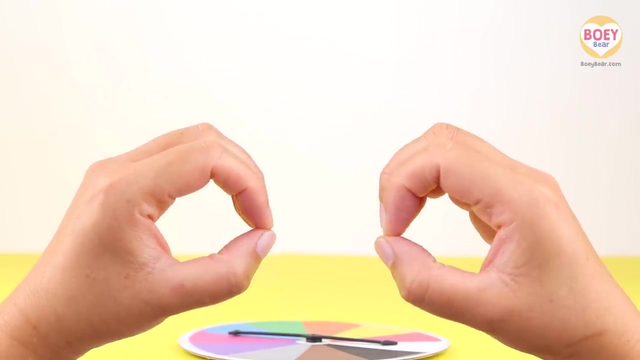 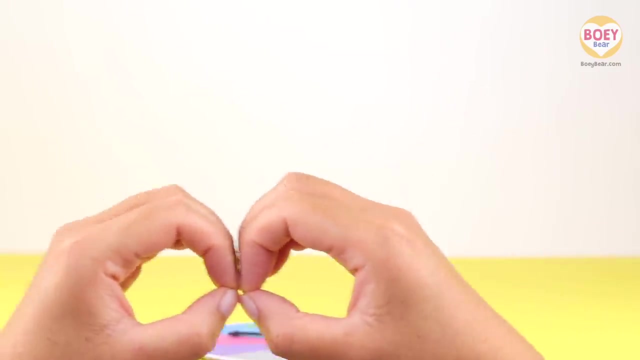 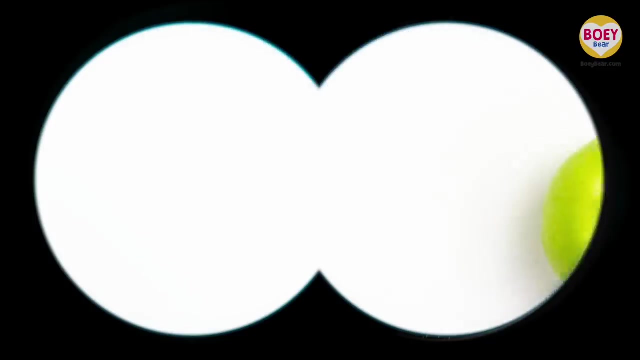 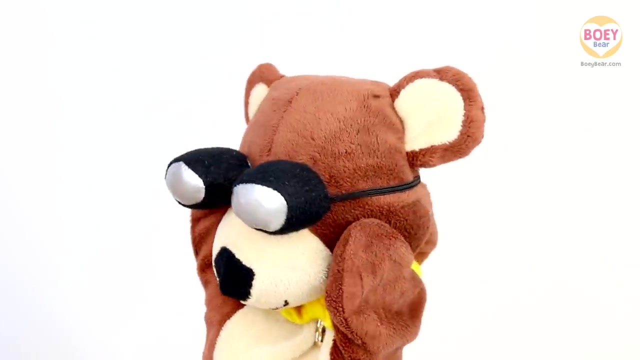 pointing to black. can you say black, black, great. make binoculars with your hands like this: put your hands together and you have binoculars from where you're sitting. can you see something, that is, have a look for today's color? what did you think of today's colour? what did you think of today's colour? what did you? 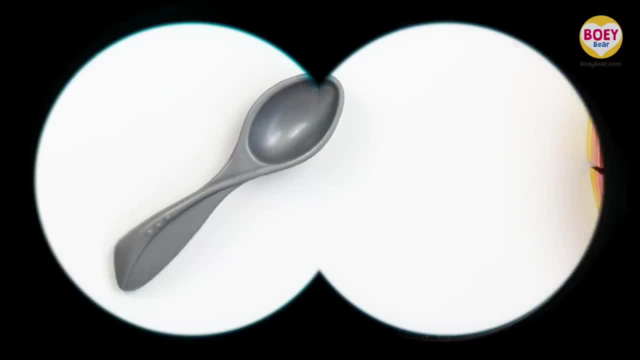 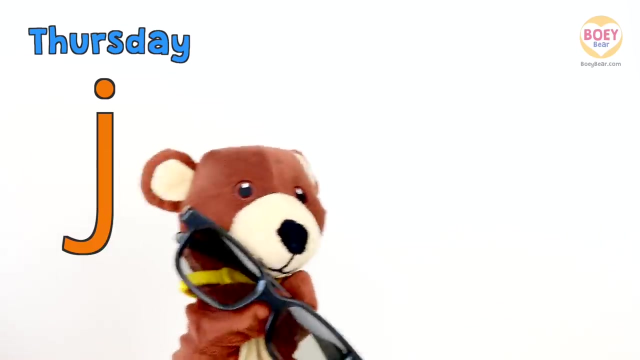 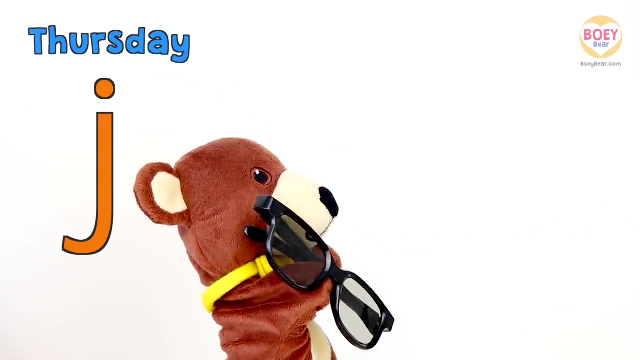 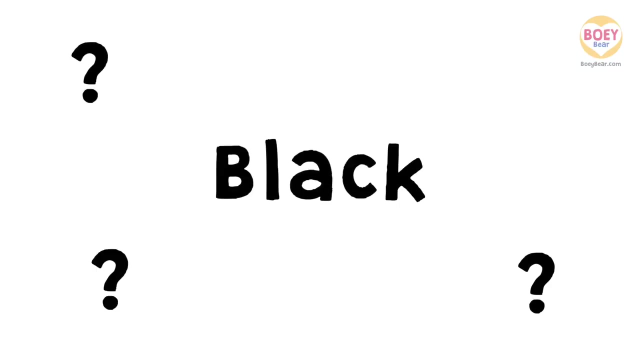 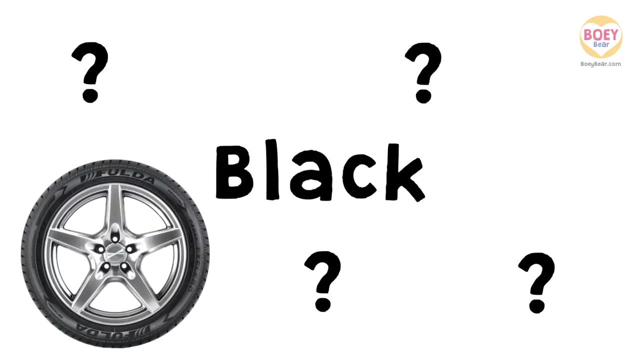 find at home. hmm, what can we see that is black? oh, what was that? these are black sunglasses. so the sunglasses, so the sunglasses. so the colour of your eyes is a little bit. colour of your eyes is a little bit. The colour of the day is black. What other things around us are black? Get ready to answer: A black tyre and a black blackbird. 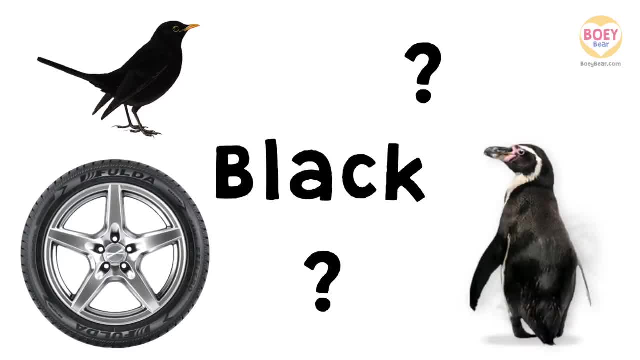 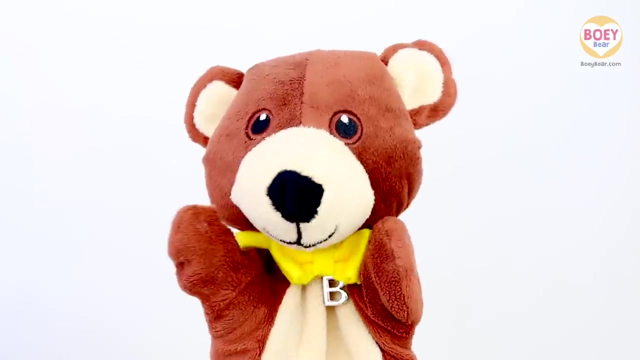 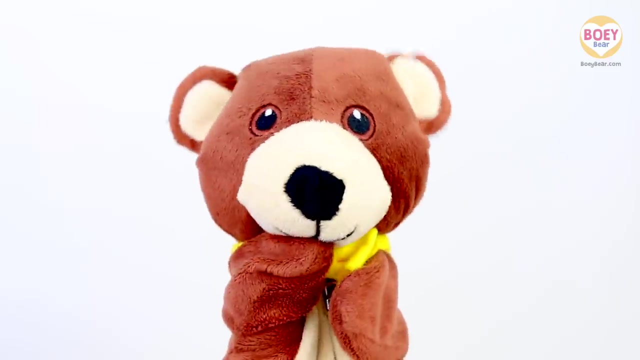 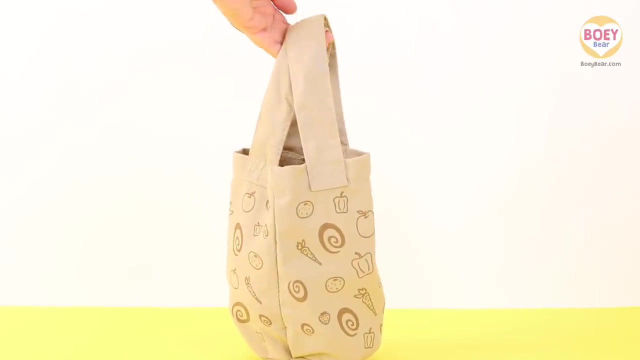 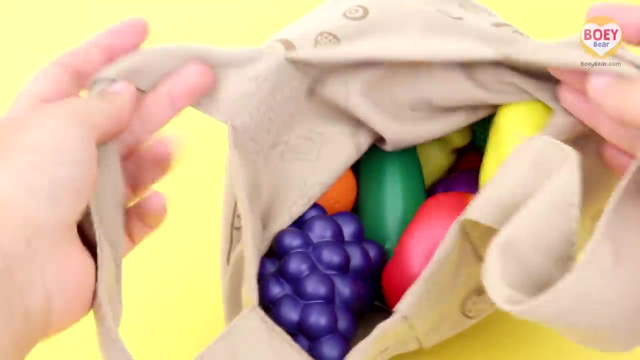 A black penguin and a black bowtie. Black blackberries, Well done. Was that your tummy rumbling, Bowie? Was it your tummy? Was that your tummy rumbling at home? Oh, it might have been mine. I think we're all hungry. It must be snack time. Here's my grocery bag. It's full of different fruits and vegetables. Have a look. 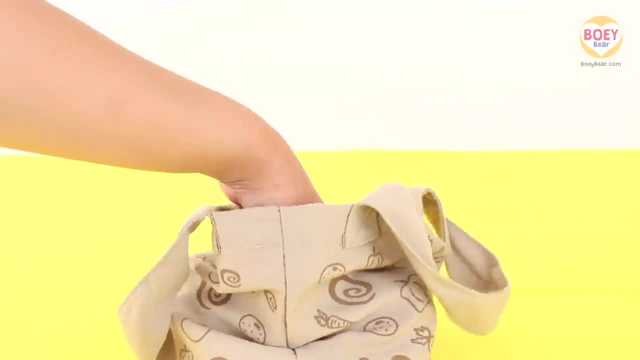 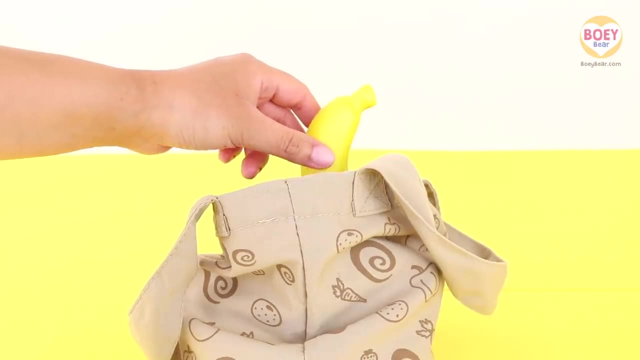 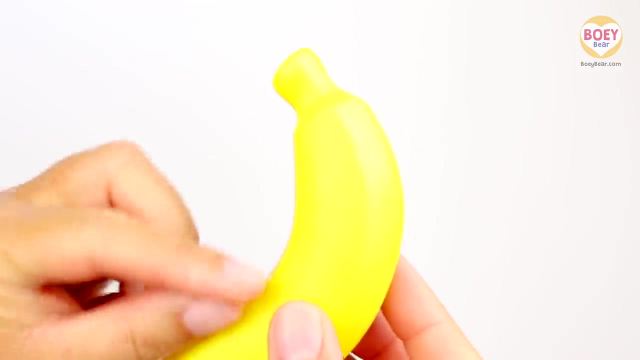 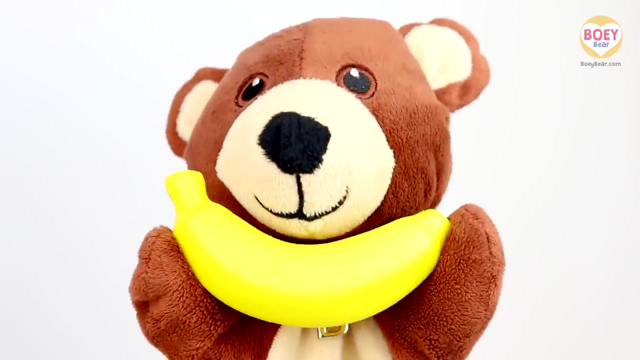 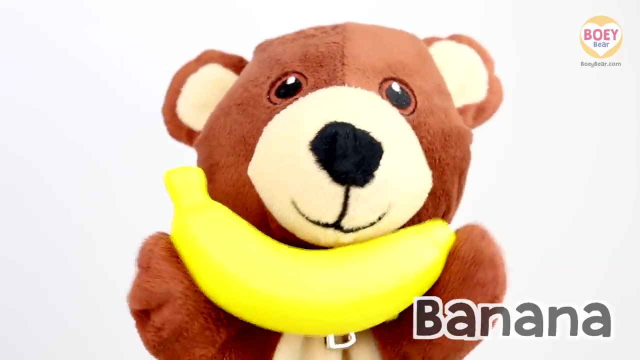 I'm going to put my hand in and pick out a fruit or vegetable for today. You have to guess what it is. It's yellow and has skin on the outside to peel. Do you know what it is? Thank you, It's like a big smile. This is a banana. 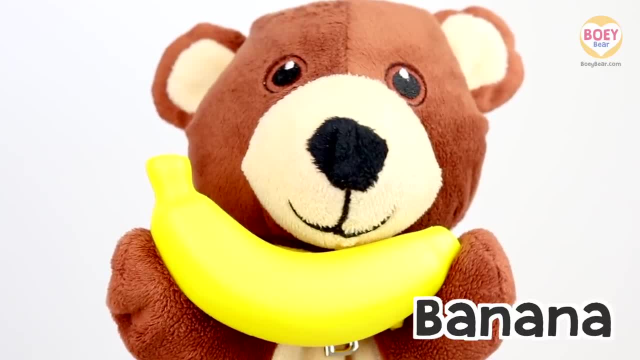 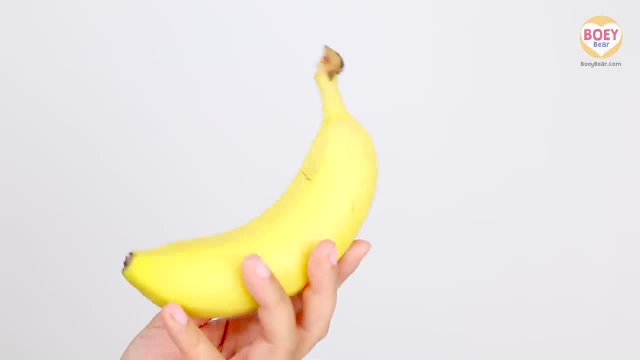 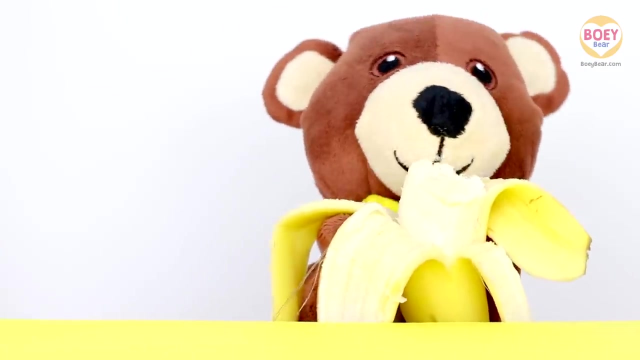 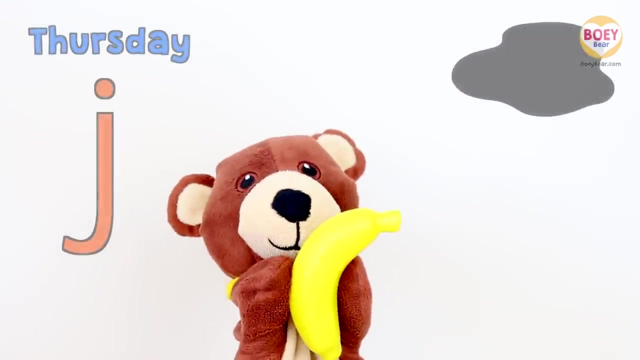 Can you say banana, Banana. Great, Let's have some bananas for our snack. You peel the banana skin like this. There you go. Yum, Yummy, It's nice and sweet. The fruit of the day is Banana. 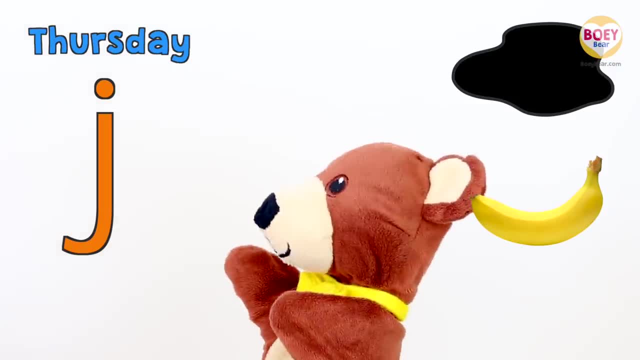 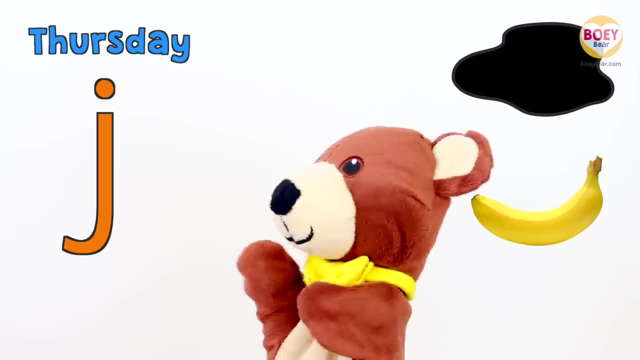 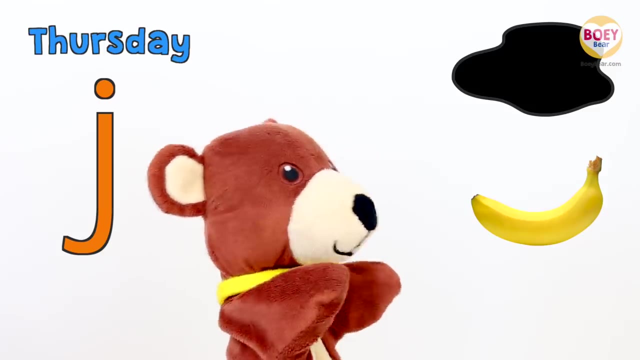 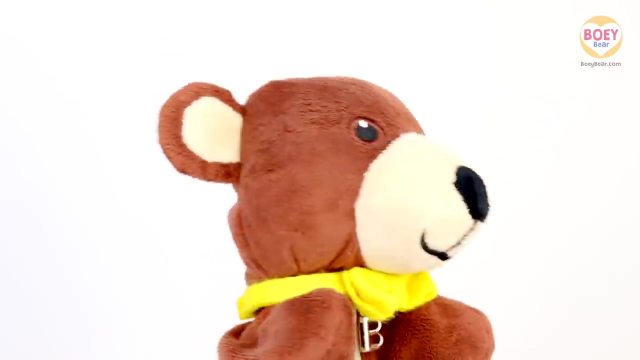 So let's go over what we've learnt today. Today is Thursday, The letter of the day is J And today's colour is Black. And what did we have at snack time? Banana. Well done, Can you hear that? A train. 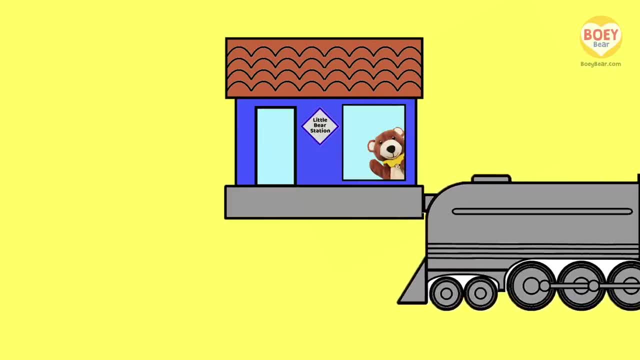 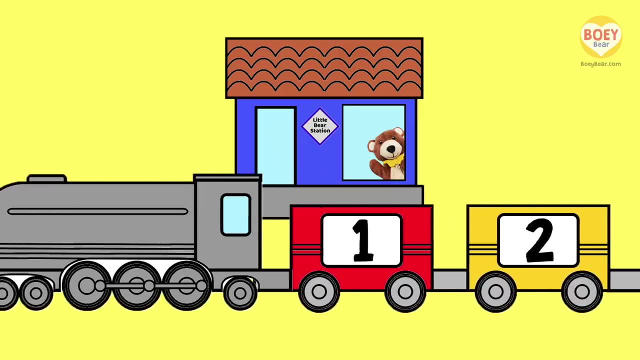 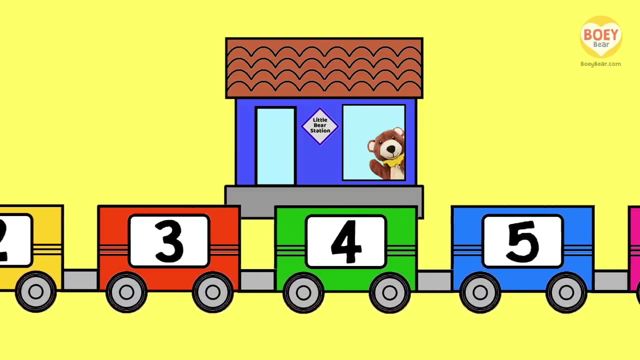 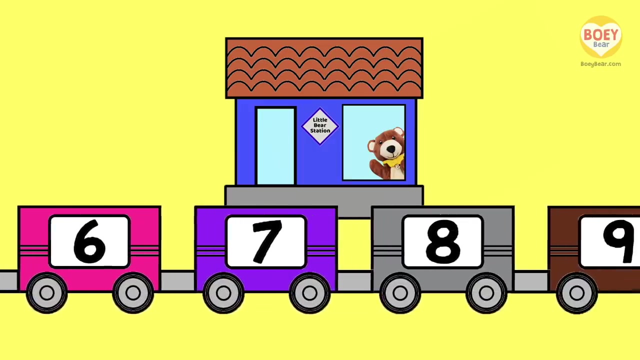 It's the number train. Let's see what number stops at the station today. Count along with me One, One, Two, Two, Three, Three, Four, Four, Five, Five, Six, Six, Seven, Seven, Eight, Eight. 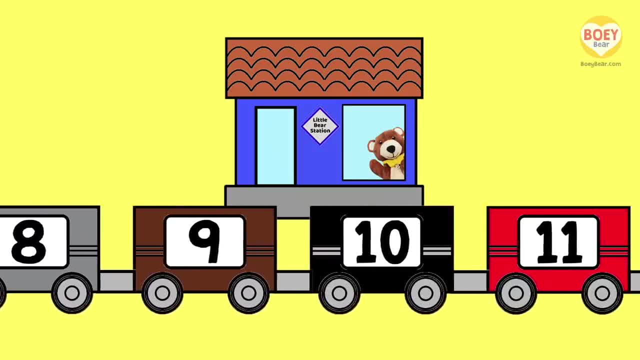 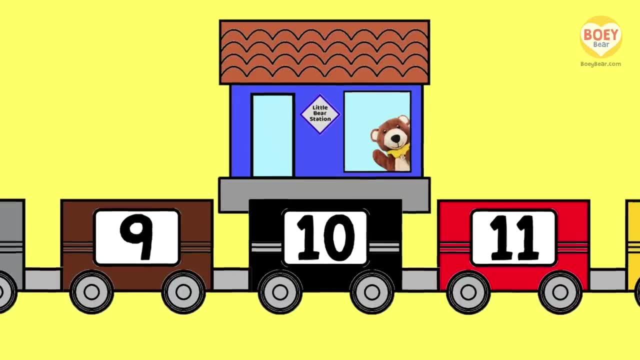 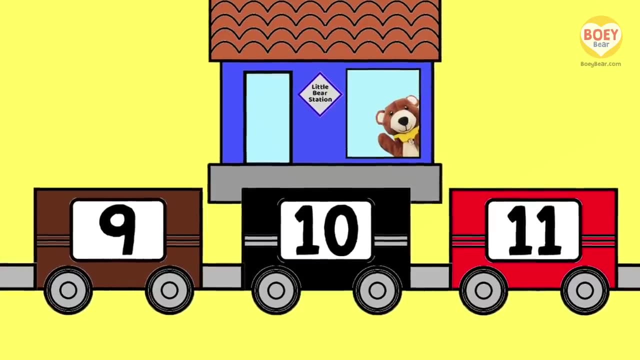 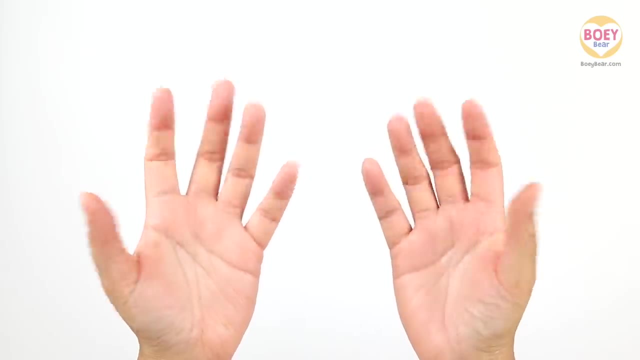 Nine, Nine, Ooh, It's slowing down. Today's number is ten. Can you say ten? Ten, Great, Now let's count the number. Put your hands out in front of you and give them a wiggle. Get ready to count your fingers. 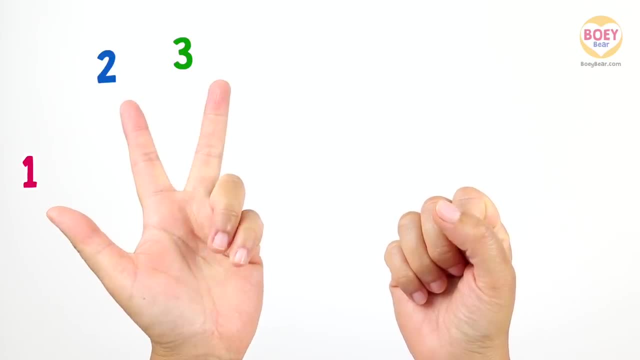 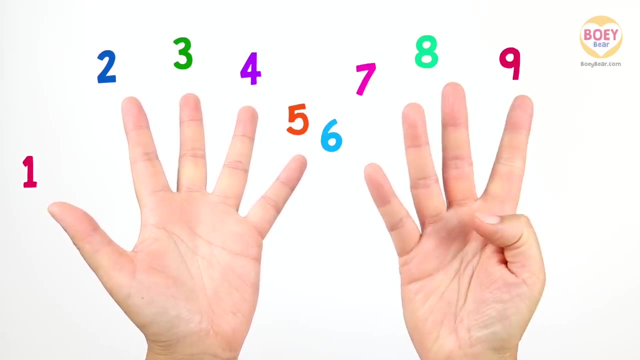 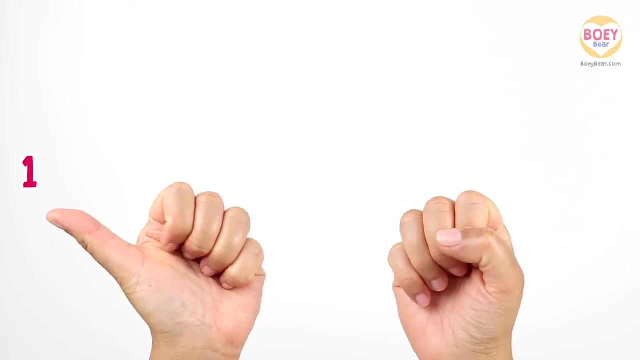 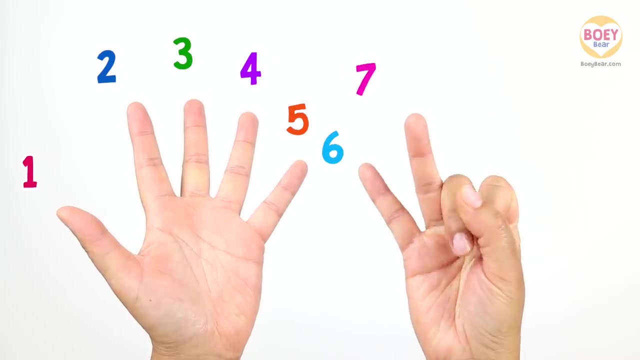 One, Two, Three, Four, Five, Six, Seven, Eight, Nine, Ten. Now it's your turn to count Ready Go: One, Two, Three, Four, Five, Six, Seven, Eight, Nine, Ten. 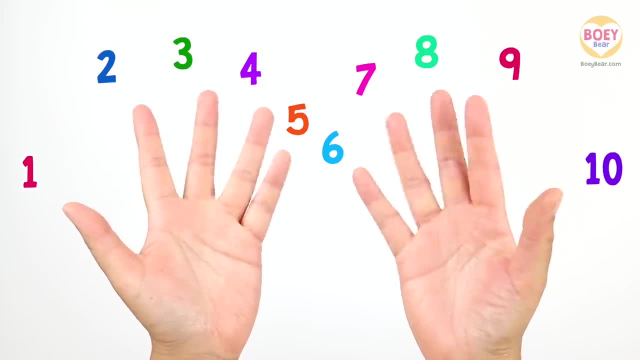 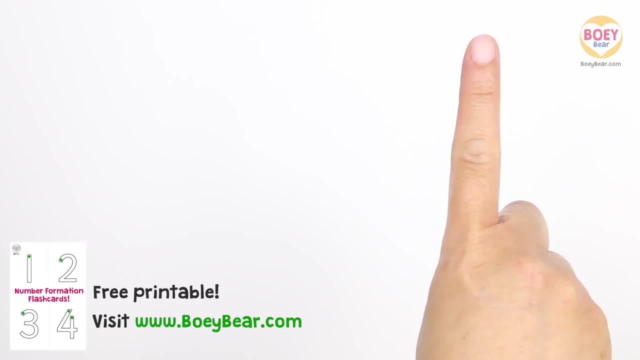 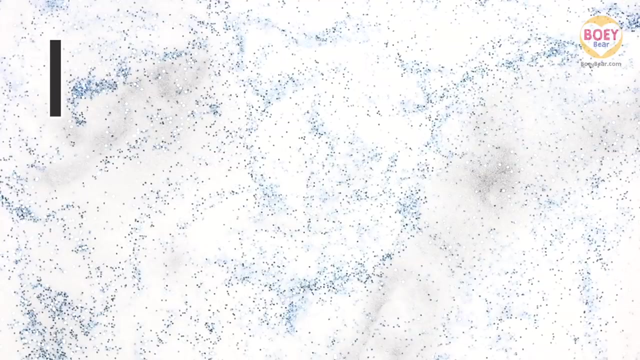 Well done, Ten fingers. Here's how you write it. Get your finger up in the air and copy along: Ready Steady, Go. The number ten is made up of one and zero. To write the one, start at the top and go straight down. 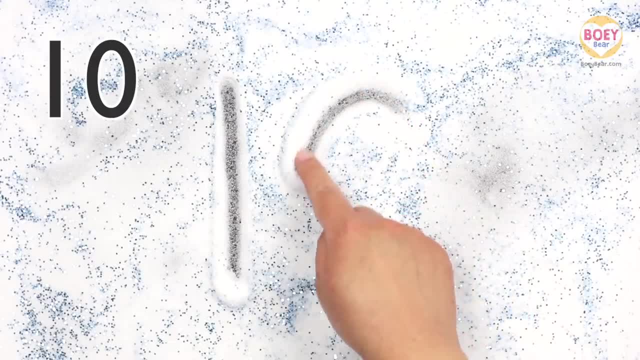 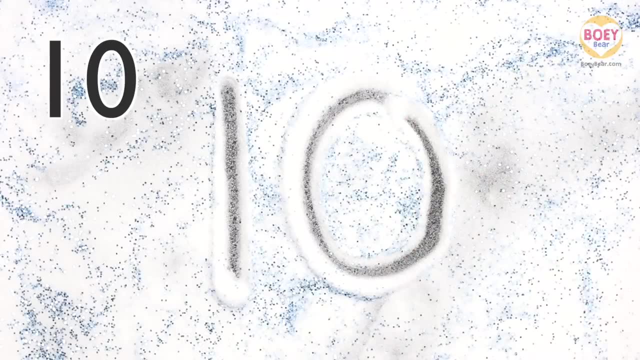 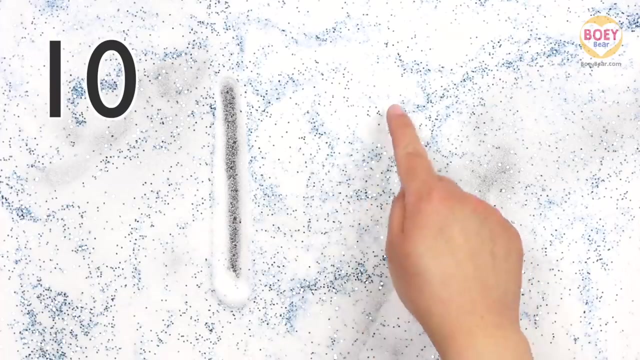 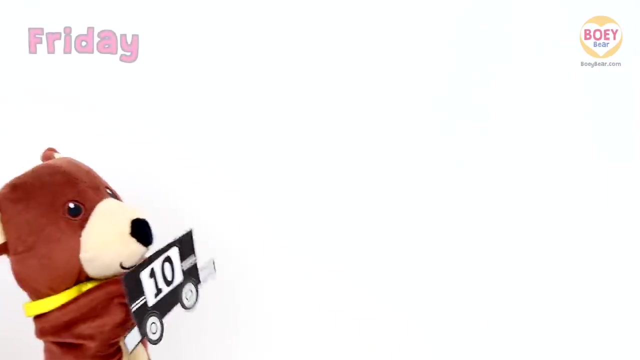 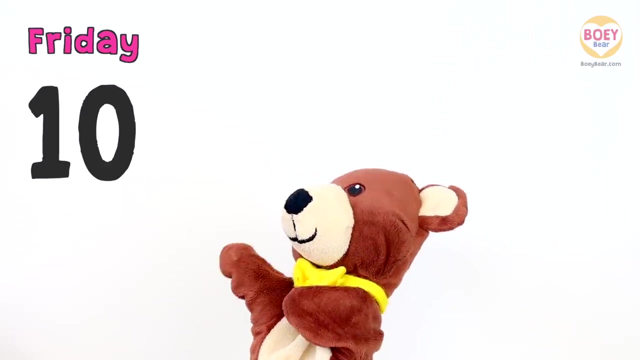 And now the zero. Start at the top, Then go all the way round. Let's do it again, but a bit faster. Copy along with your finger in the air: Well done. Today's number is ten Ten One, Two, Three, Four, Five, Six. 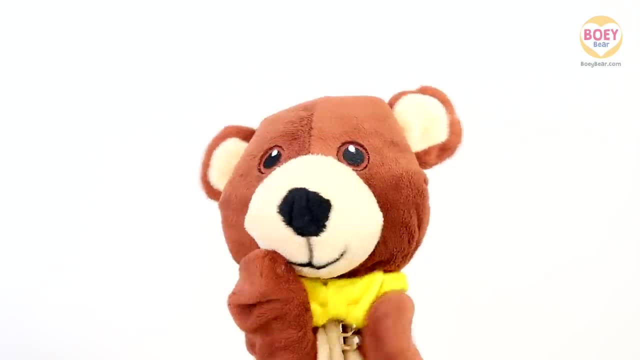 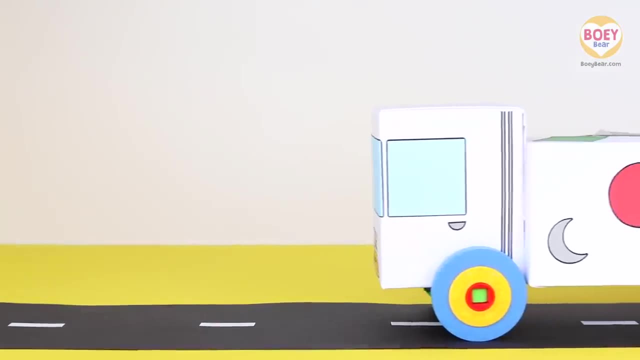 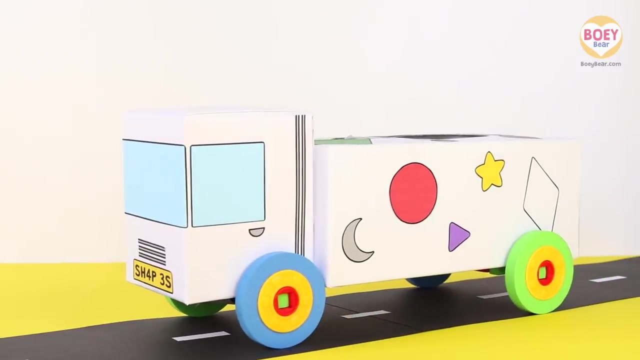 Ten One, Two, Three, Four, Five. Six One, Two, Three, Four, Five, Six Great. Can you hear that? What's that? It's the shapes truck. This is the shapes truck. I wonder what shape is inside. 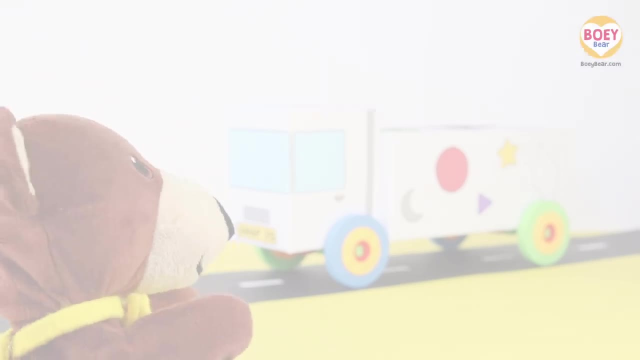 I'm going to put my hand in it. I'm going to put my hand in it. I'm going to move my finger like this: What shape is inside? I'm going to put my hand in and see what shape we have today. 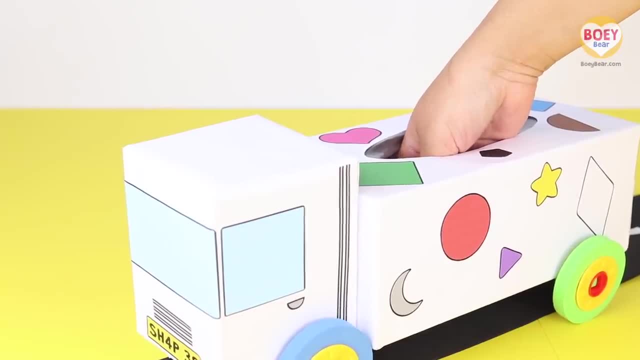 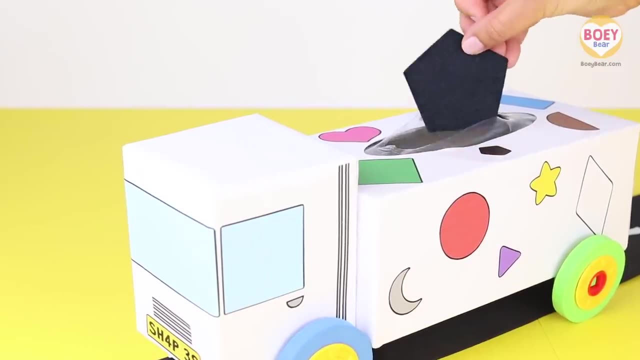 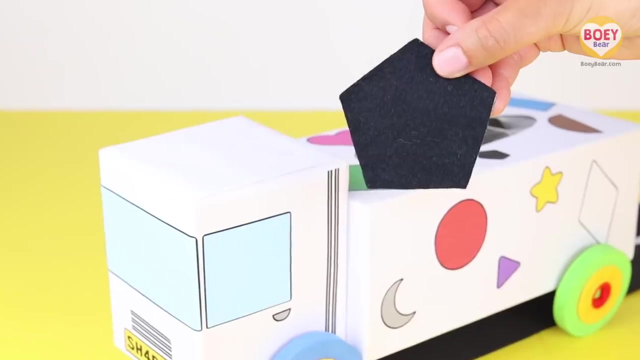 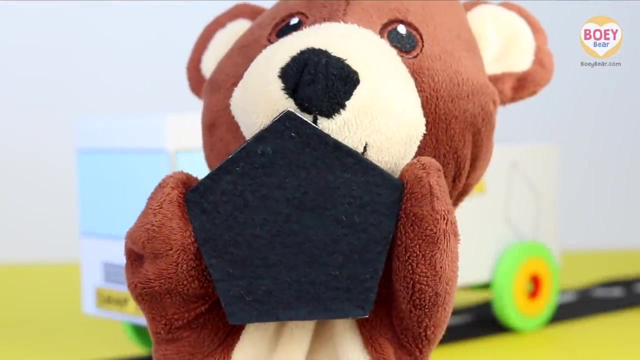 Hmm, it has five pointy corners. Can you guess what shape it is? It's a Pentagon. Can you say Pentagon, Pentagon, Well done. It has five pointy corners: One, two, three, four, five corners. 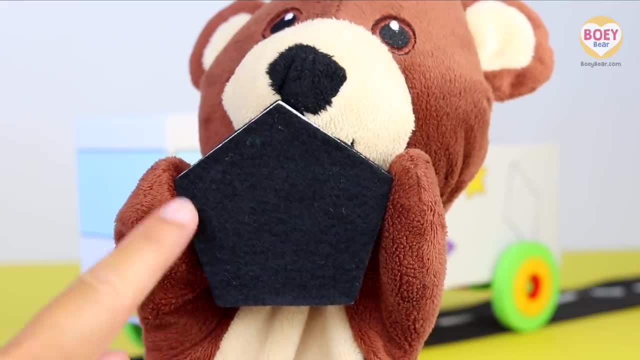 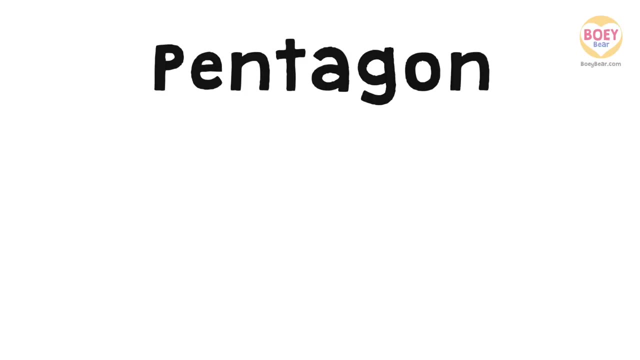 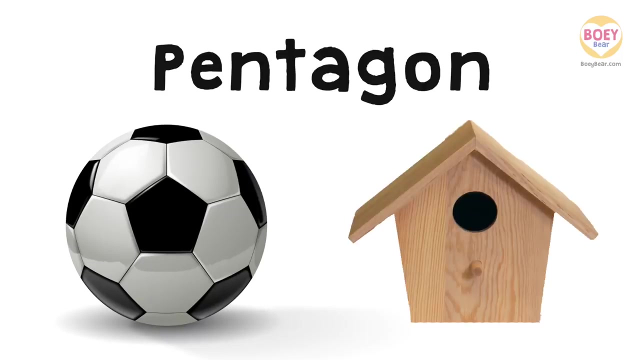 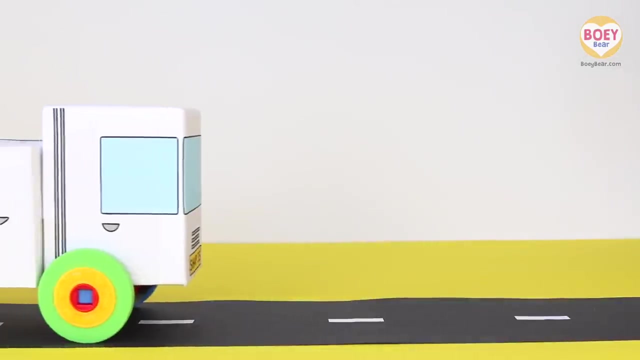 And five straight sides. One, two, three, four, five sides. What things around us are Pentagon? Get ready to answer. Pentagon shapes on a Football, A pentagon-shaped Birdhouse. Great, Thank you, Shapes Truck. 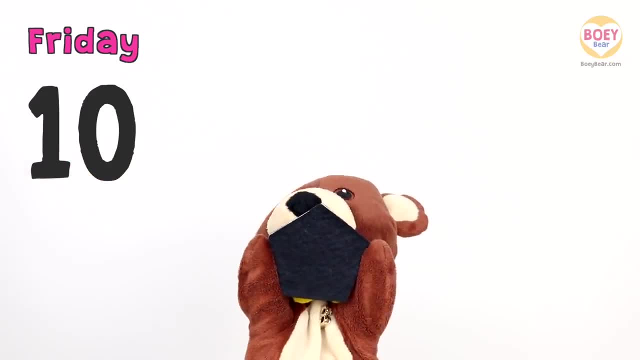 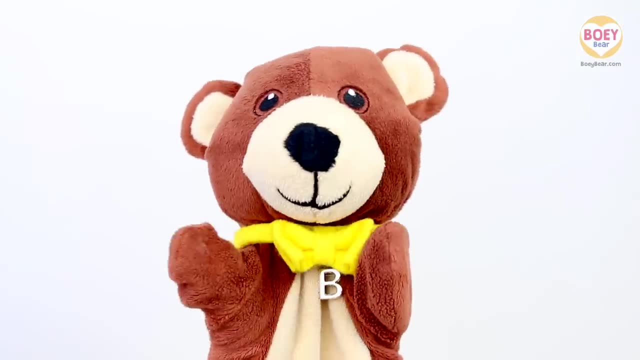 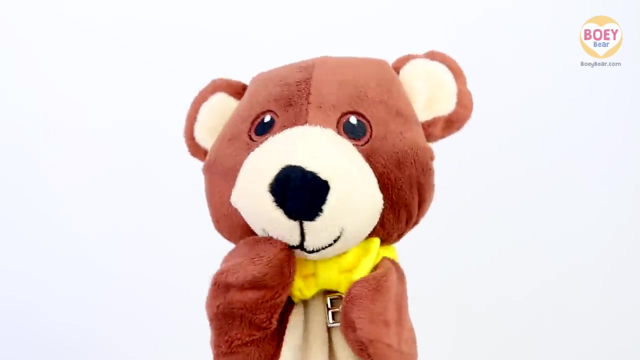 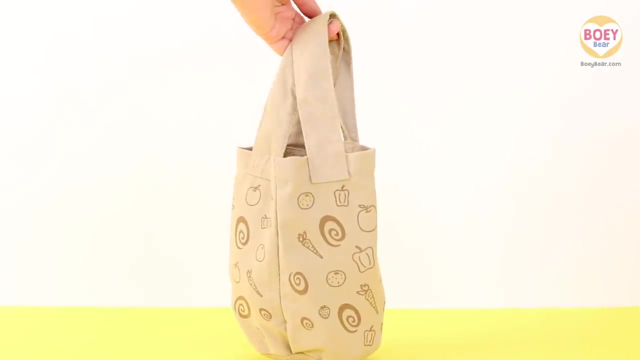 So today's shape is a Pentagon. Pentagon, What's that? That's your tummy rumbling, Bowie. Was it your tummy at home? Oh, it might have been mine. I think we're all hungry. It must be snack time. 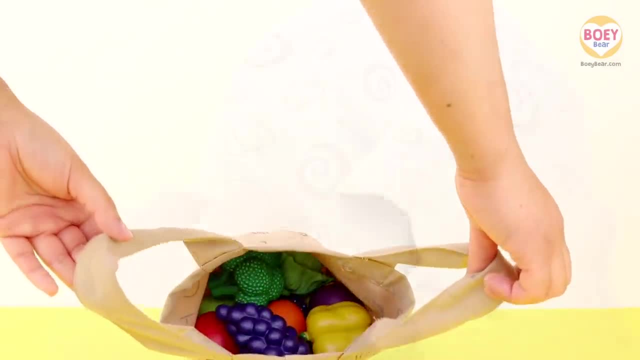 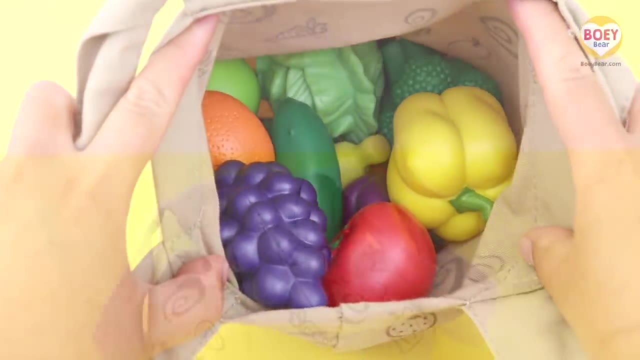 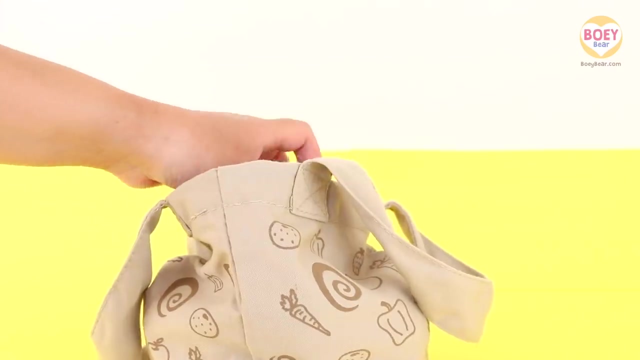 Here's my grocery bag. It's full of different fruits and vegetables. Have a look, I'm going to put my hand in and pick out a fruit or vegetable for today. You have to guess what it is. You have to guess what it is.